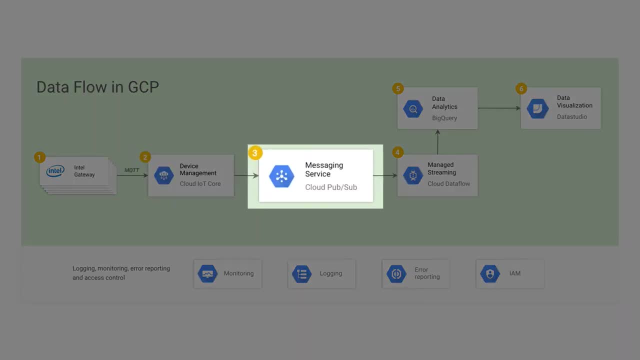 IoT Core. That data ends up in a PubSub queue. From the PubSub queue we'll use a Cloud Dataflow pipeline to take that data from the queue into a durable storage service called BigQuery And from BigQuery we'll visualize that data using Cloud Data Studio to create 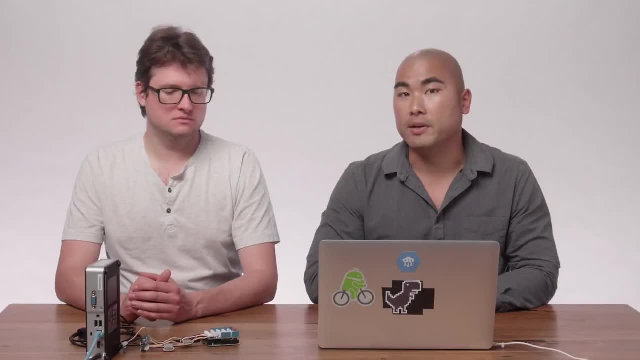 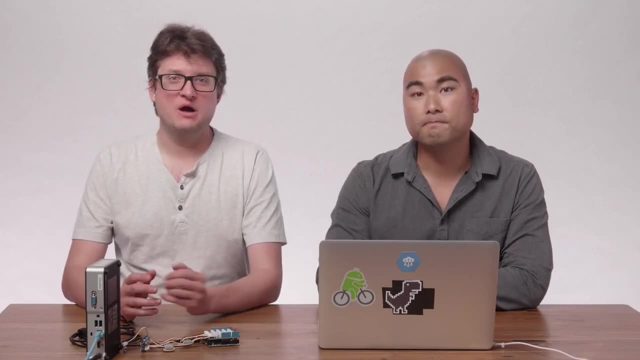 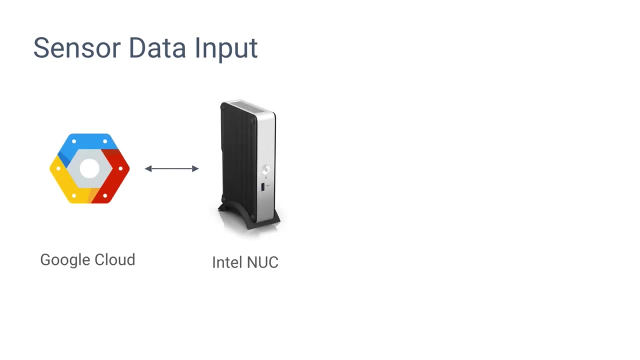 wonderful dashboards, But before we dive in, let me throw it back to Martin to talk about the hardware setup. Sure, So I just want to take a quick look again at how the sensor data is actually getting into GCP. So for this demo, we're using the sensor data that's coming from our 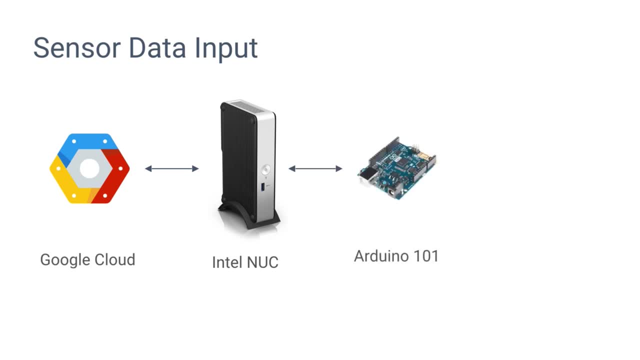 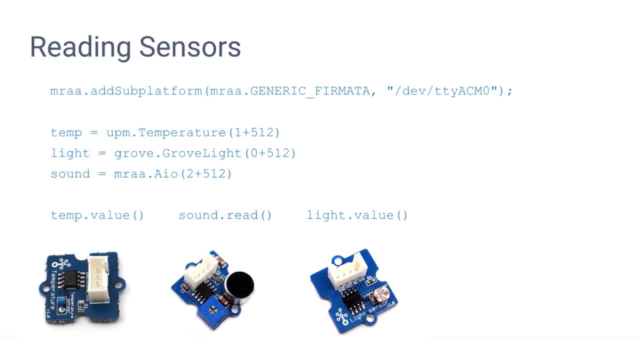 gateway here And we have our gateway attached to an Arduino 101, which we're using as a sensor hub. Attached to this hub are three environmental sensors- temperature, light and sound- In order to read the sensor data we're using. 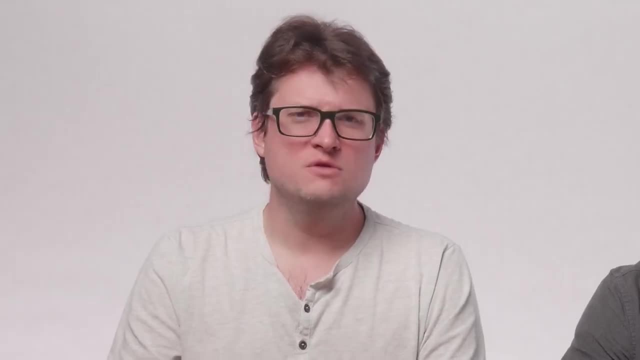 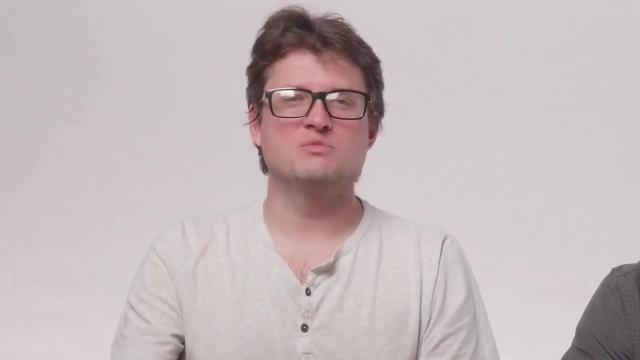 the EMRA and UPM libraries from Intel. We can use a really simple high-level API to connect to the sensor hub and then read out our values from the sensors. If you want to learn more about these libraries and how you can use them, please refer back to the first. 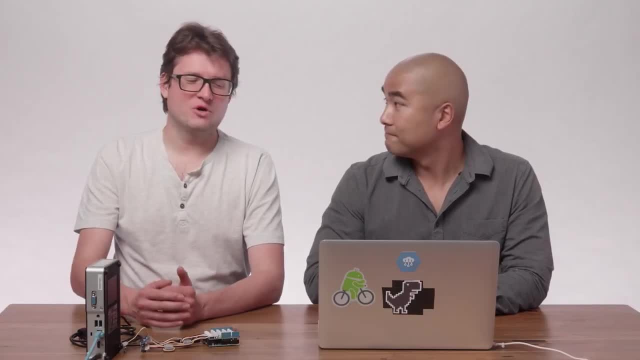 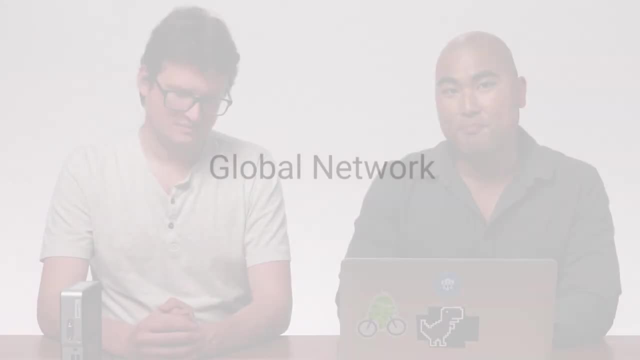 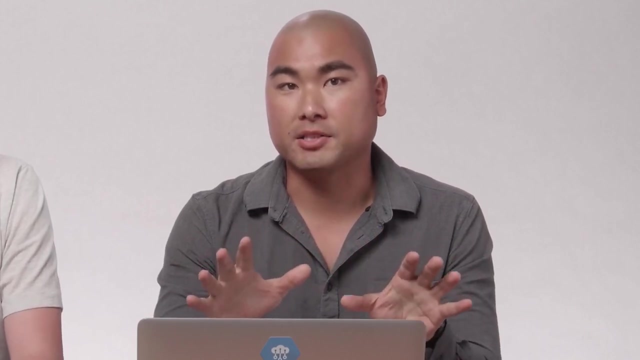 webinar of this series. So, Josh, do you want to tell us a little bit more about that data journey? Absolutely, Before we begin, I'd like to take a minute just to explain a little bit about our global network. Now, this is important because your devices could be deployed all over the world And 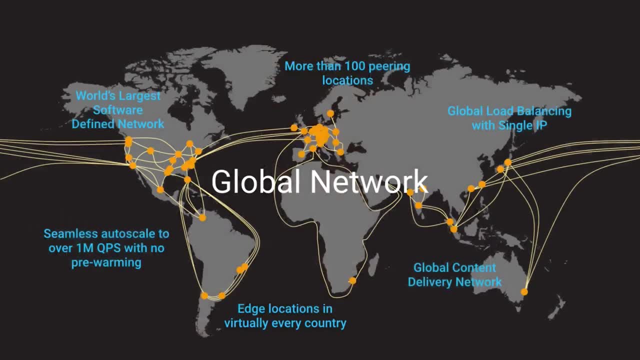 this has implications in how your devices communicate back to the cloud. What you're seeing here is a map of our global network. You'll notice we have over 100 peering locations. What this means is that, most likely, we'll have a presence in the country where your 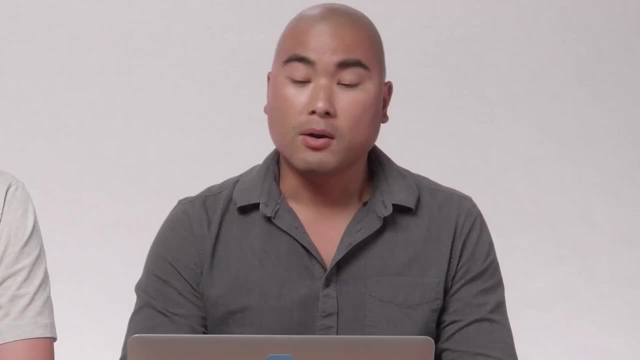 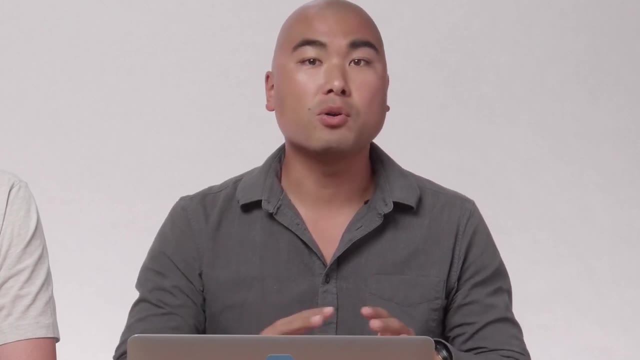 devices are deployed into. This also means that, with a single global IP address, you could send all your data to that single IP address and Google will automatically load that data to your device. And that's what we're going to do today. So let's get started. 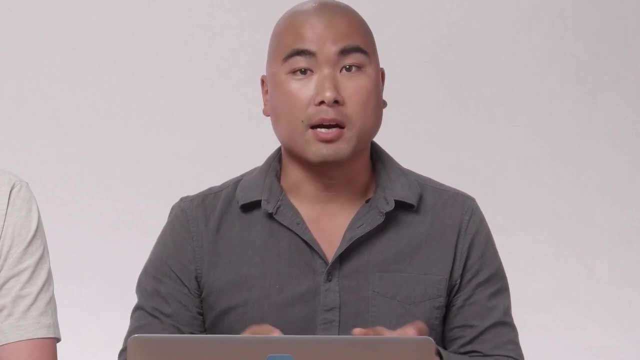 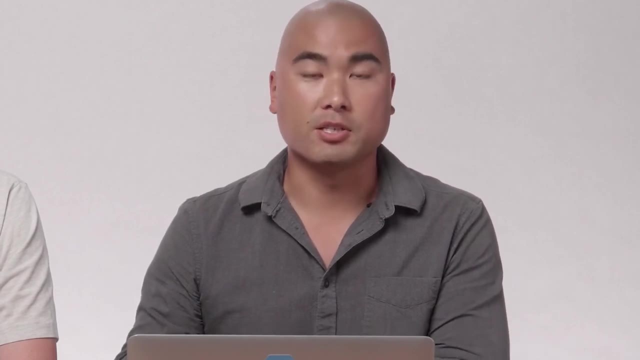 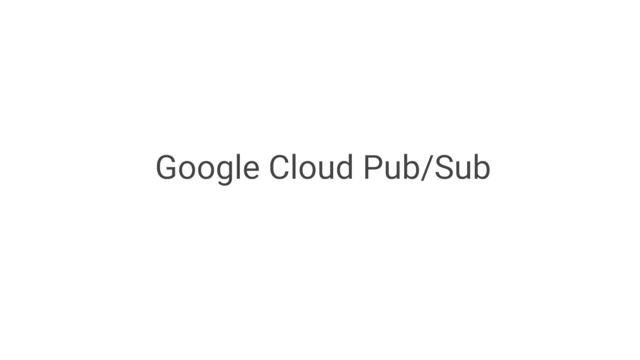 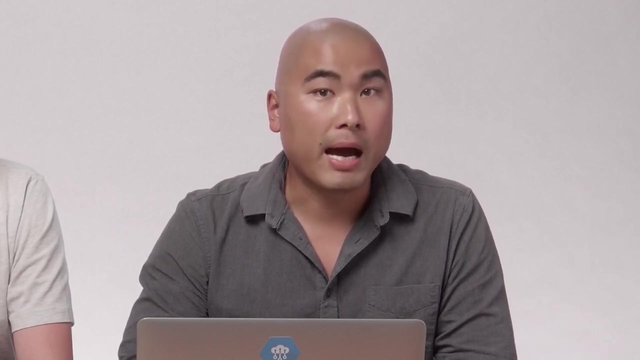 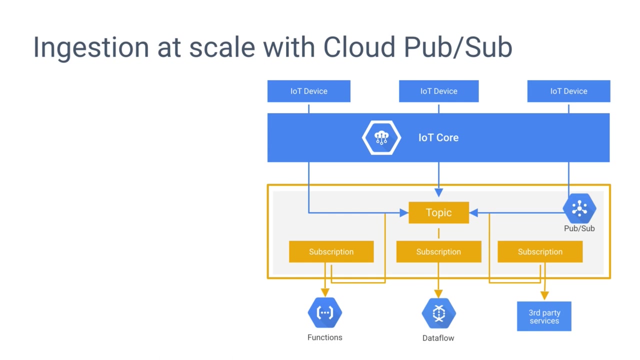 Let's get started. Let's talk about the first service to explore on our journey, and this is PubSub, our globally distributed, highly-scaled messaging service. When data is sent to Google Cloud IoT, it ends up in a PubSub topic. Multiple subscribers can subscribe to these topics and retrieve. 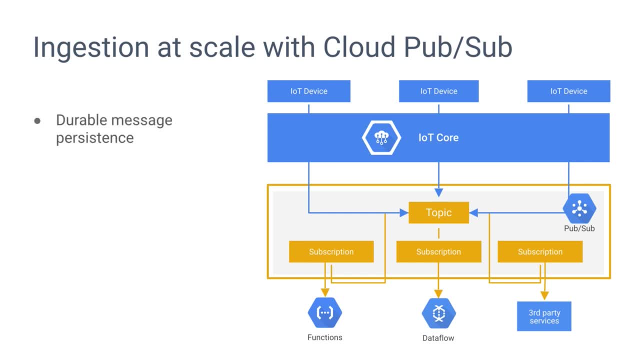 information. It's a durable service, meaning we will retain unacknowledged messages for up to seven days. It's a global service as well, meaning you could write to a single URL or IP address and Google will handle the load balancing for you, Coupled with either. 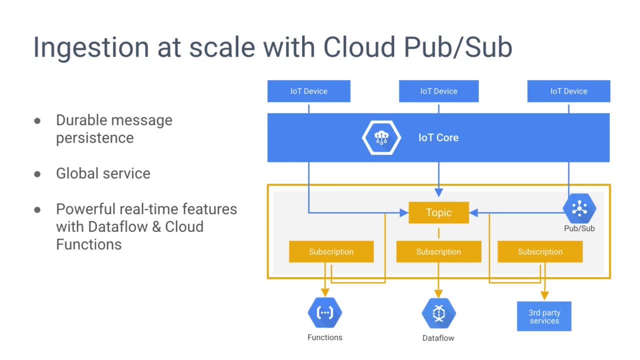 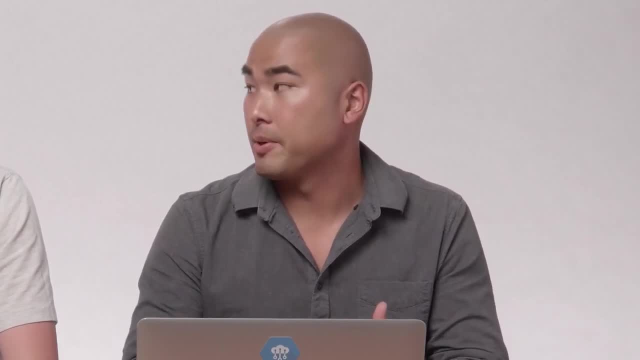 data flow or cloud functions. PubSub is your on-ramp to real-time streaming into the cloud. Let me demonstrate how easy it is to set up your own topic. I'll also set up a simple subscription. So what you see here is the Google Cloud PubSub user interface To get there on your 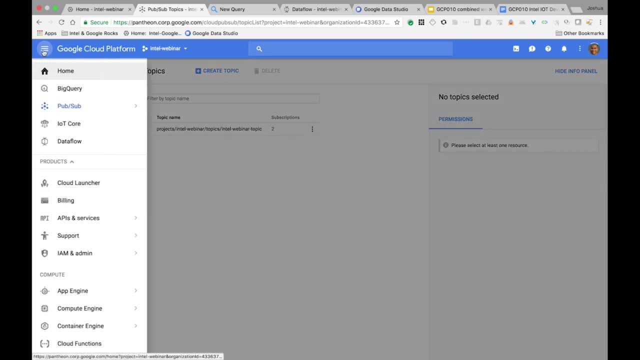 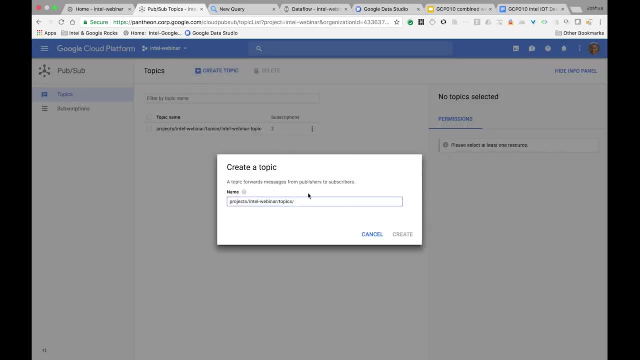 GCP landing page. you would simply click on the hamburger menu and select PubSub To create a topic. you would select Create a Topic and then define your own topic. In this case, let's just call it Demo. Click on Create And just that easy. you created a topic, but 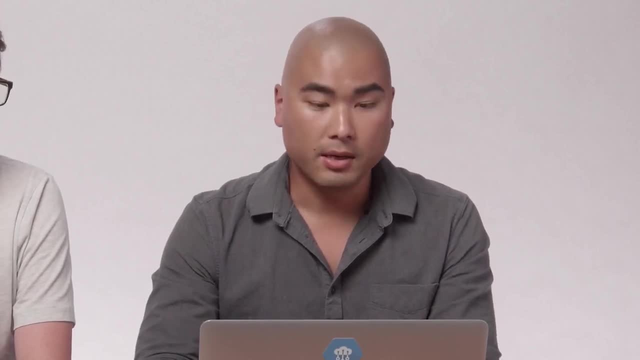 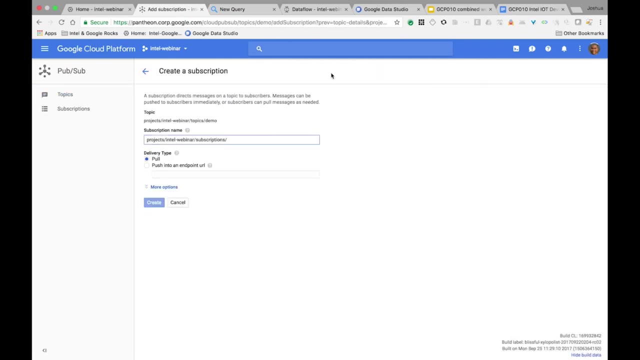 doesn't really do anything useful until you can create a subscription. To create a subscription, simply go into the Demo topic and click Create. You can create a subscription for that, If that you just created, and then click on create subscription and this case we'll. 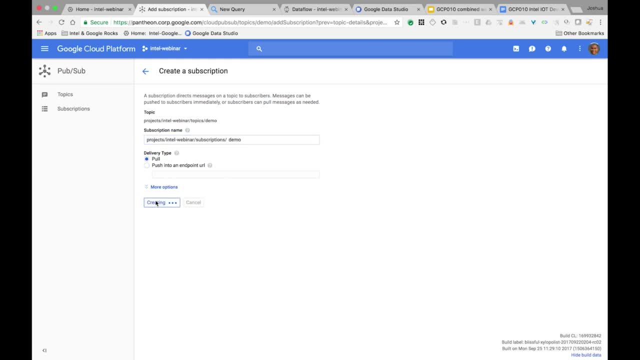 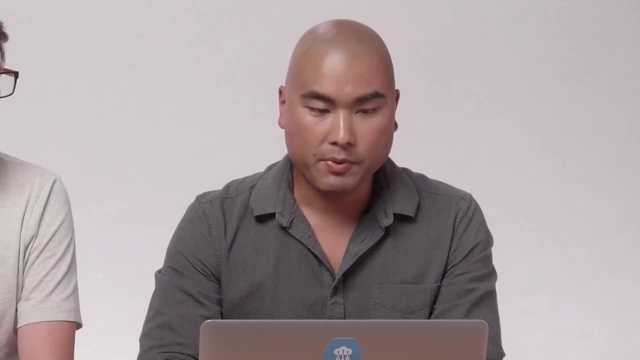 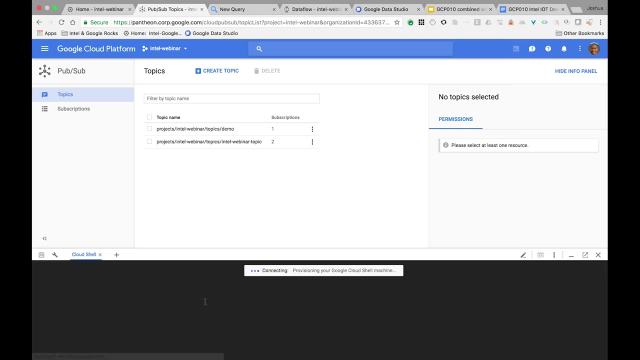 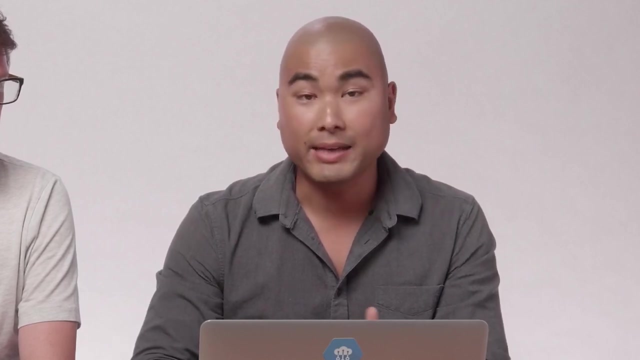 just call it demo and there you have it. you have your first topic and subscription duo, so let's do something useful with this. now. we've been sending data from the endpoint here into PubSub. let's see what that looks like. okay, and in this case I will issue the simple gcloud command to pull data from that. 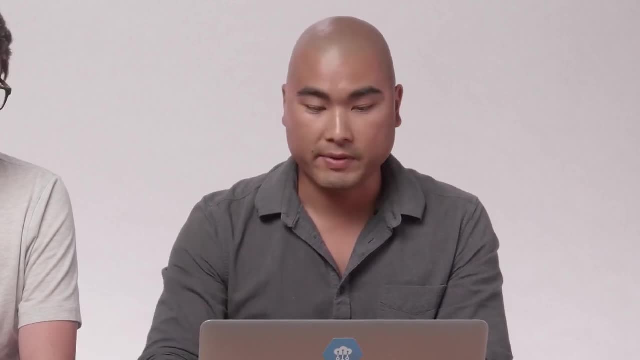 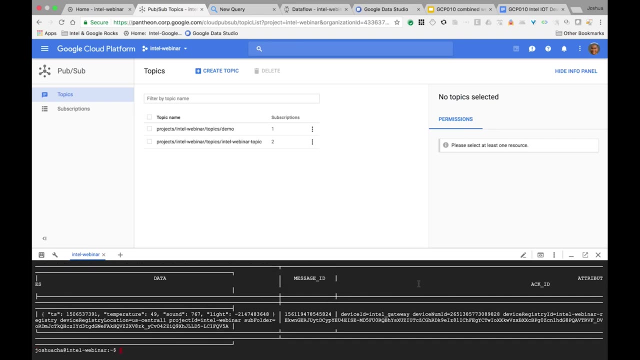 subscription or to an existing subscription. I had that, received the data from the endpoint and there you go. this is the data being sent from the sensors to the nook, to through IOT cloud, through PubSub, and there you have it in the subscription. yeah, pretty straightforward. 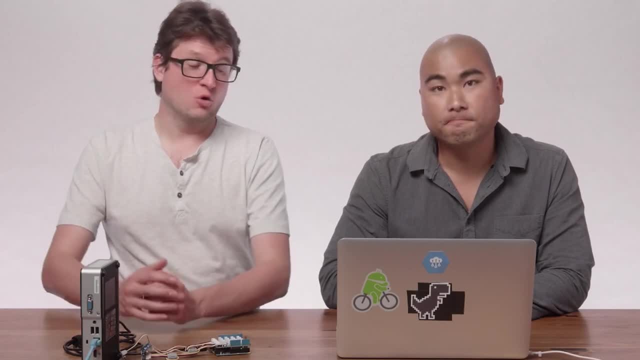 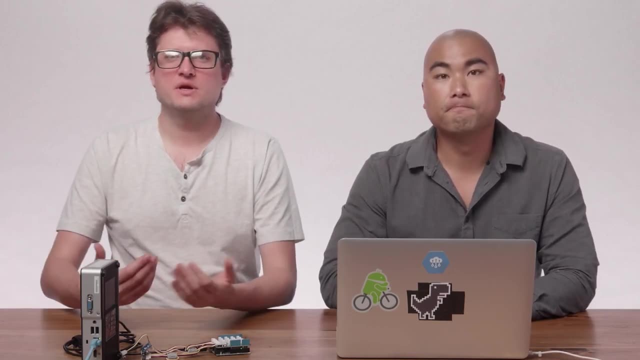 you know, Josh, you talked about scaling up your data infrastructure using the global GCP network and, as you scale up the cloud, in the back end, you're also going to want to scale up your harbor deployments in order to gather more sensor data, be able to enact any commands that you want to send down. 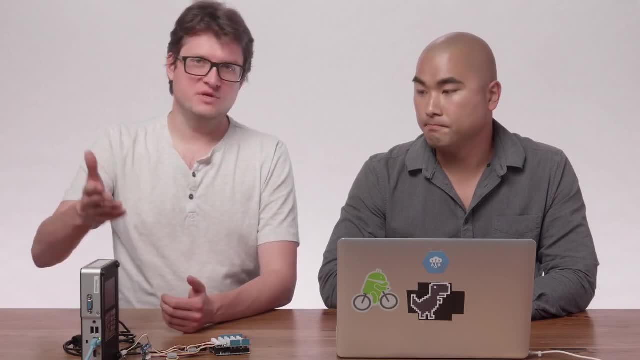 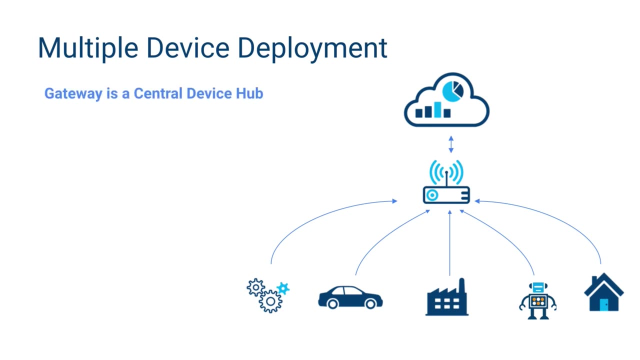 so, as you do this, having a gateway is going to be key. so the gateway acts as a central hub for all the sensors and actuators in a local area. you can send the data gathered from any number of sensors using any kind of interface. for instance, if you're scaling out your data from a local network, you can send data from any kind of interface, for instance, if you're scaling out. 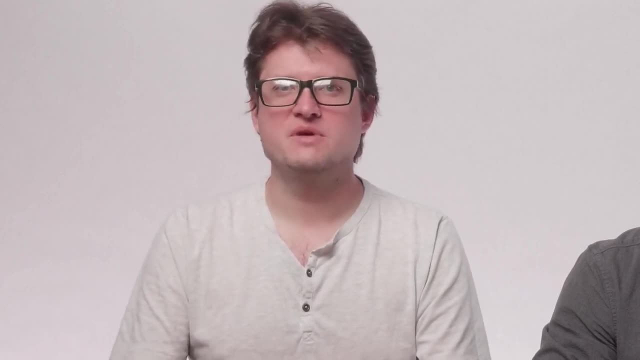 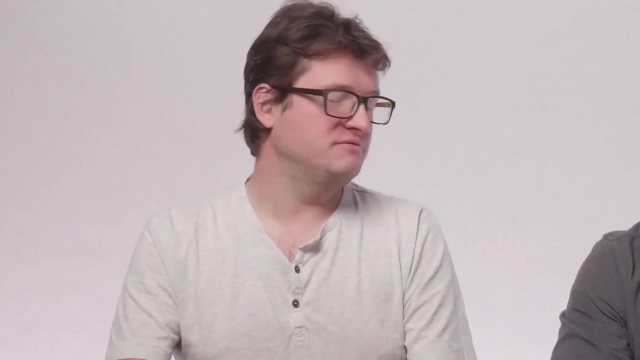 to a factory that has a lot of Legacy sensors, by which I mean sensors that do not have a way of connecting to the cloud themselves. you're going to need a device that can't connect to the cloud and act as a data collection and communication hub, so Intel has Gateway Solutions that can interface with. 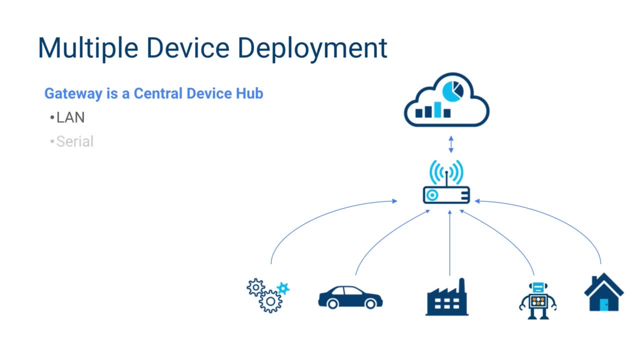 sensors over the local area network or using a serial connection like Modbus or cambus, or short-range radios like Bluetooth, Zigbee or z-wave, as well as many more connection types. so by having a single connection point to the cloud, you're going to inherently increase the security of your deployment. you limit possible points of intrusion. 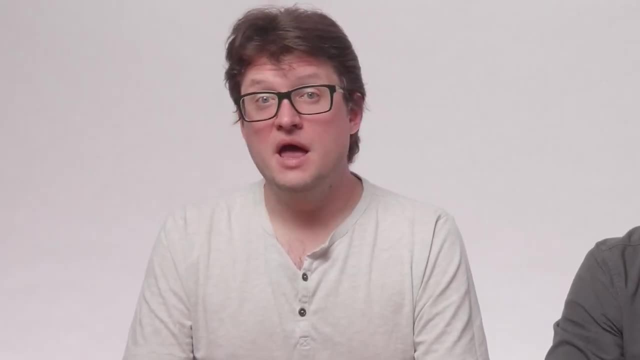 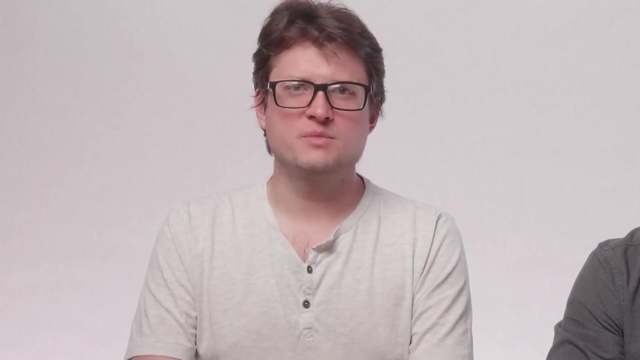 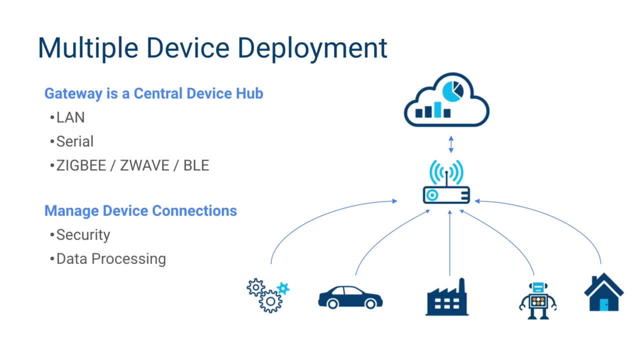 they're going to limit the number of certificates you have to manage and you can use the Gateway to set up a firewall that only allows certain protocols through using an IP table. overall, it's going to be much more secure than trying to manage a multitude of connections. you can also run some data pre-processing at. 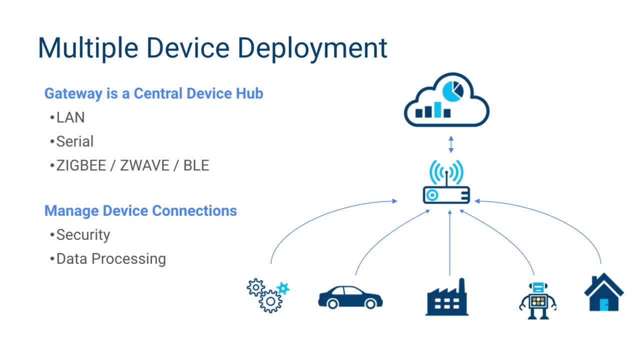 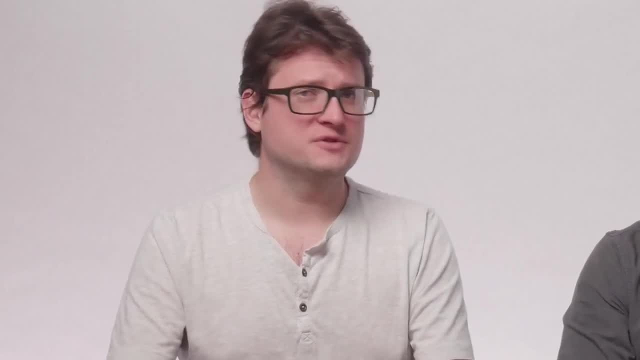 the Gateway before shipping it to the cloud- basic things like taking an average over time to much more complex data transformations, and I'm going to come back to this point a little bit later on with a few examples. finally, as the scale of your data increases, you're going to want to also make sure that 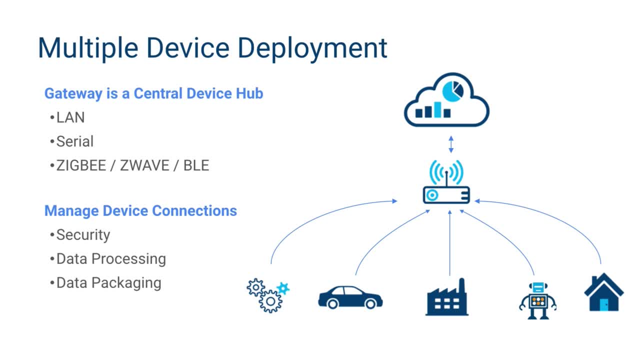 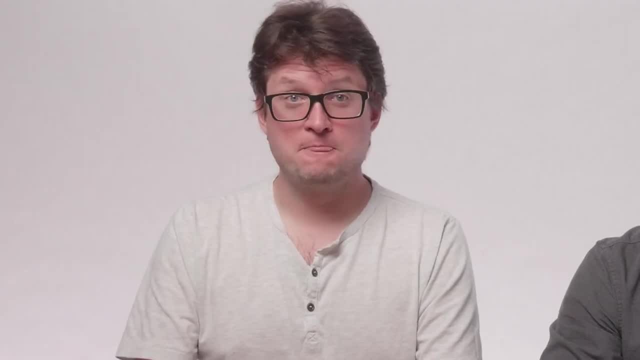 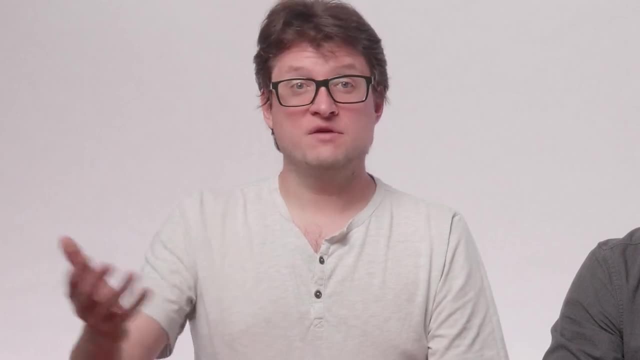 it's consistent. so consistent data is going to be easier to parse as well as to manage, and the gateway can also package up that data for consistent cloud ingestion. so in our case, and in many cloud connection use cases, we're using JSON to send the data back and forth, so this data transfer method is easy for humans to read. 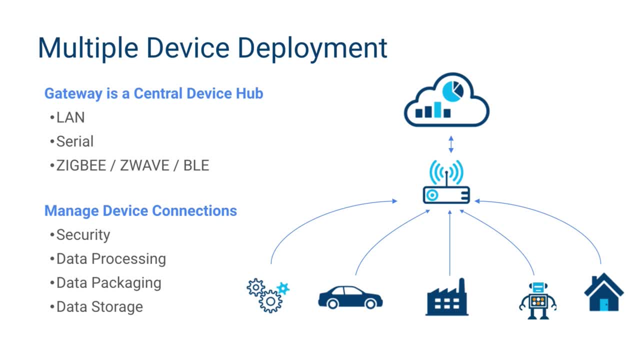 and it's easy for machines to parse. it's also quickly becoming a standard for IOT data transport, so you'll be able to interface with many different services using the same data pipeline. another aspect of scaling out your project is scaling out the scope of what the project itself 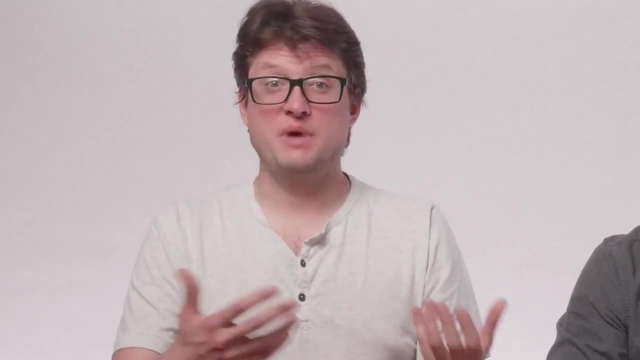 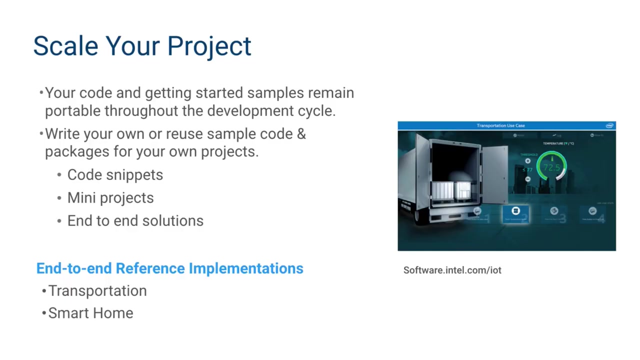 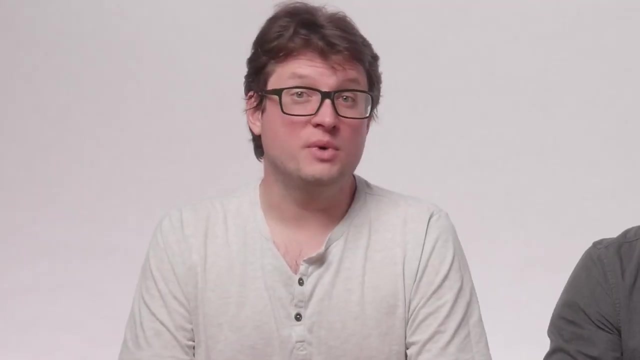 can do so in order to help developers really expand the capabilities of their projects. we have at Intel what the path the product provides is code samples, proof of concepts, as well as market research into specific verticals in the IOT space, including smart home, transportation, autonomous driving, so on. it's all open source and it's all up on GitHub under MIT licensing, so you can use what. 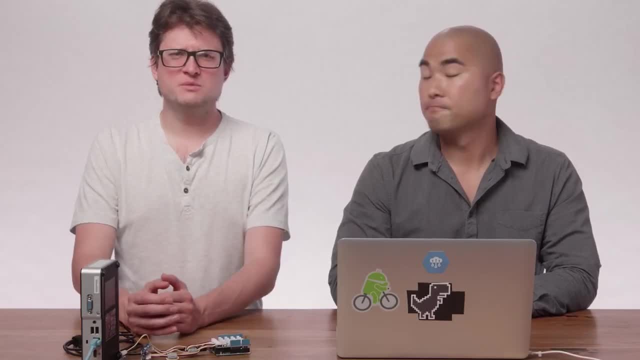 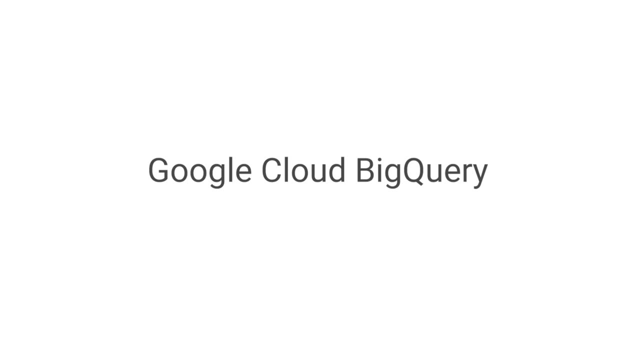 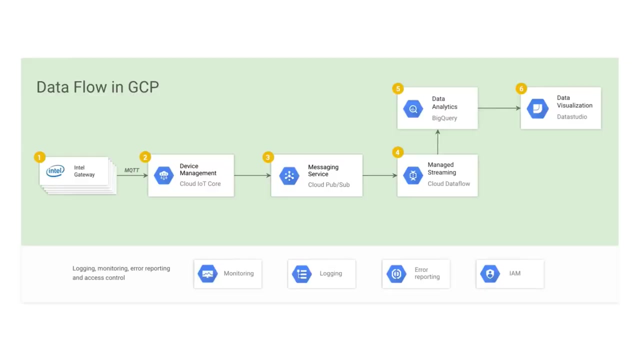 you need from our code. Josh, do you want to tell us a little bit more about what the data can do in BigQuery? absolutely so. BigQuery is my favorite GCP product. now in the journey, you'll see that we're going to skip over data flow and we'll get back to that in a second. you'll see why. for now, let's talk about 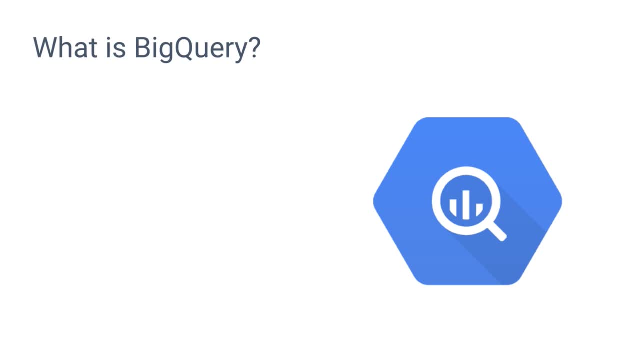 BigQuery. BigQuery is Google's analytics database that's built for petabyte scale. it's ideal for the analytics use cases because you don't have to worry about deploying more resources when you're constantly pumping in more IOT data from these devices. it's fully managed: no ops data. 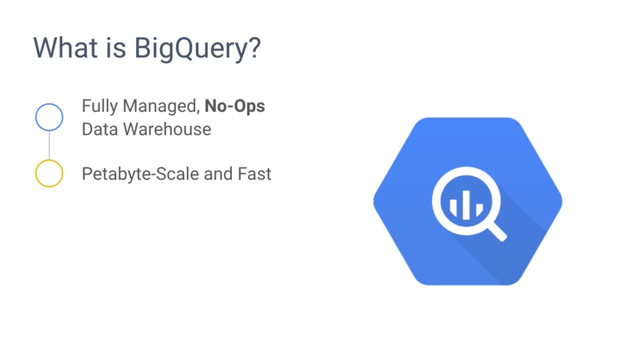 it's built for petabyte skills mentioned- but it's super fast. at the same time, you get the convenience of SQL, so if you're used to writing SQL, you'll be able to work with BigQuery easily. and finally, it's an externalized version of Google Dremel, which is a database we've been using internally. 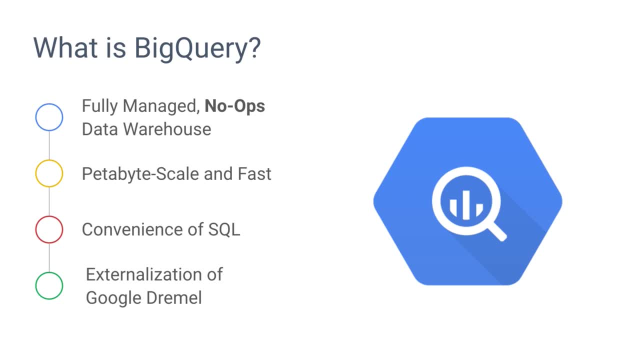 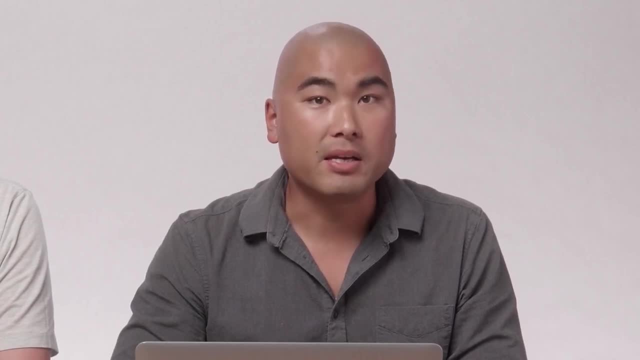 for over a decade. so it's been hardened, it's been tested and it's been put into production for well over 10 years now. so let me demonstrate how easy it is to set up your own database and issue some simple commands. so what? the first thing you'll notice is that you 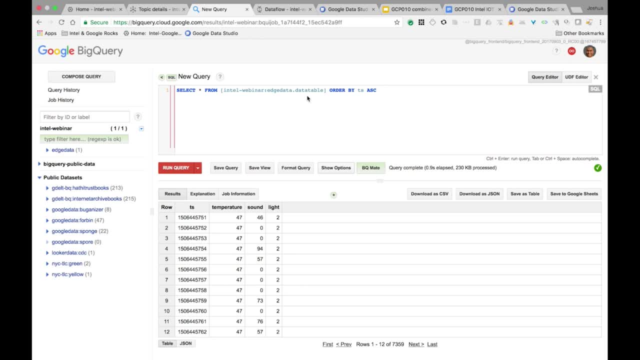 you're using SQL constructs here, so you're going to select star from this table. order by ascending order. click on one creator. it's going to run the query and notice how fast it was. this table has over 7 000 rows. let's try it in descending order. run the same query to see the data change a bit. 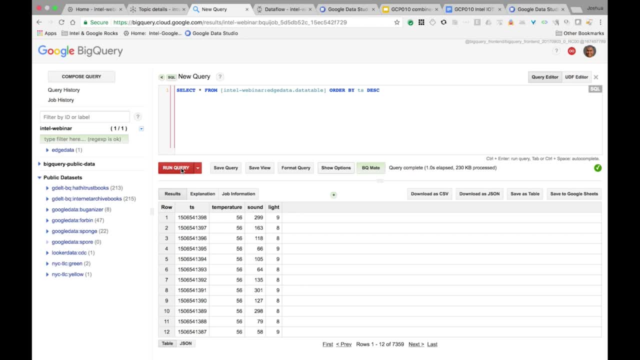 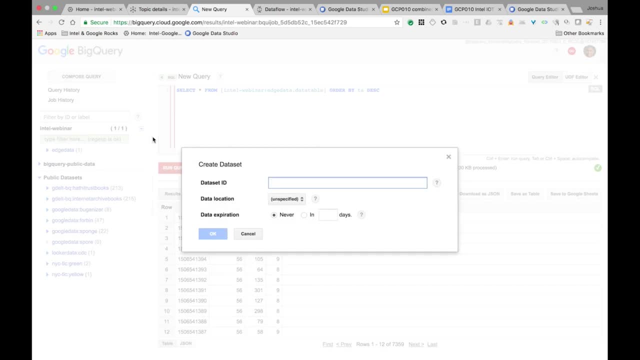 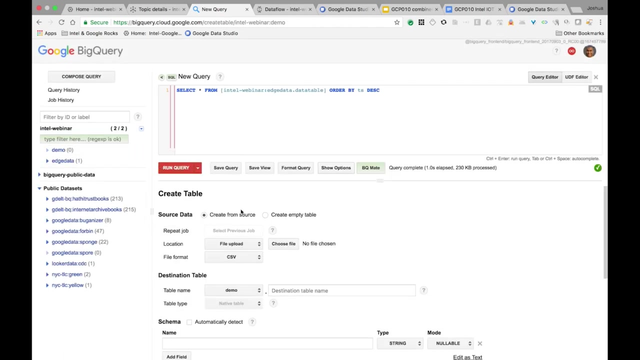 and there you go, right. so it's going to sort this in descending order. notice how super fast it was to create a table. again, click on this down arrow, super fast. we're going to create a data set. we're going to call it demo. click on okay and from the demo you can create a new table. see, and you can either create from: 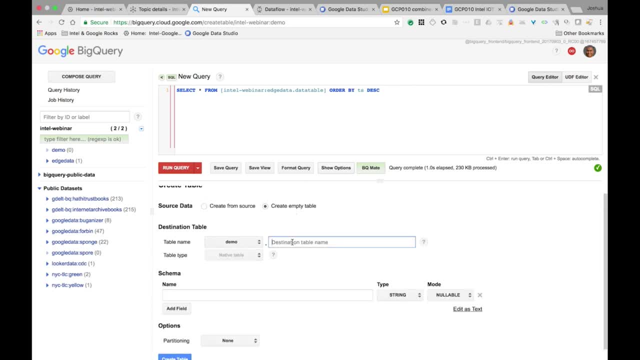 source or create an empty table. let's just create an empty table and call it demo table. keep that in mind- we'll get back to that in a little bit- and just add a couple fields. let's try timestamp, which is an integer, and let's try temperature, which is a float here. so I'm 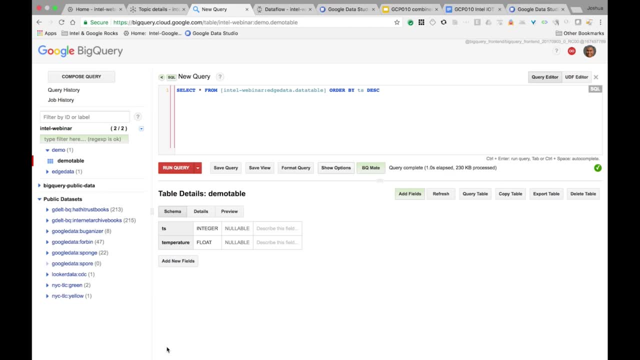 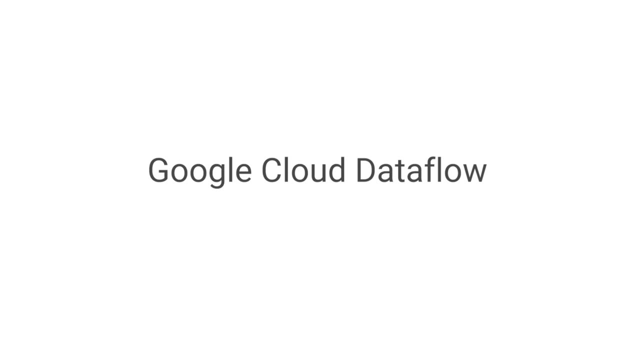 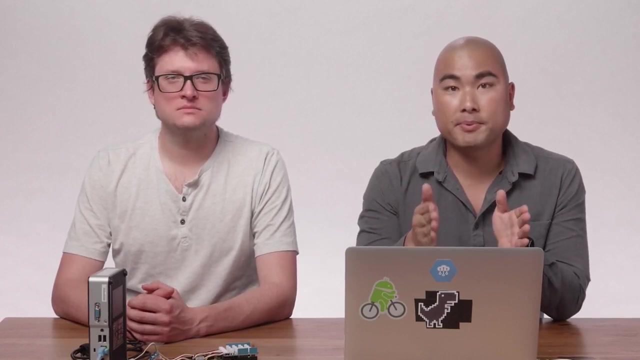 going to click on create table and there you have it, your first BigQuery table. now that we have data coming into PubSub and we have a place to store that data, how do we get that data from the PubSub topic into BigQuery? there are a few options, but today we'll focus on cloud data. 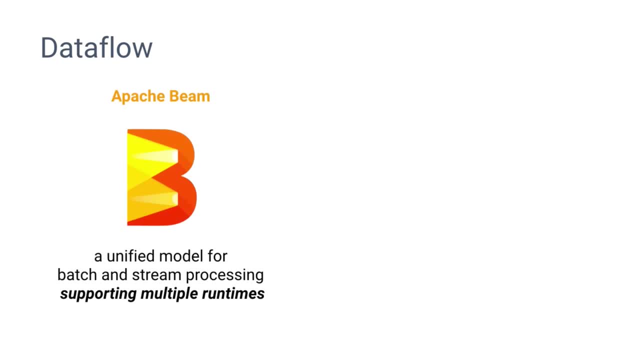 flow. if you are familiar with Apache beam, then you'll feel right at home with cloud data flow. cloud data flow is a fully managed service for transforming and enriching data in stream or real time or in batch historical, so no more complex workarounds or compromises needed at a high level. you define a source which 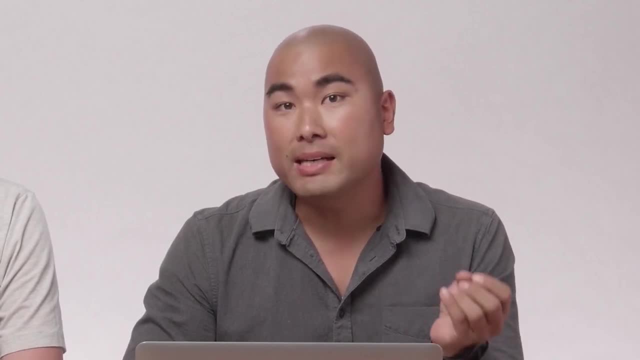 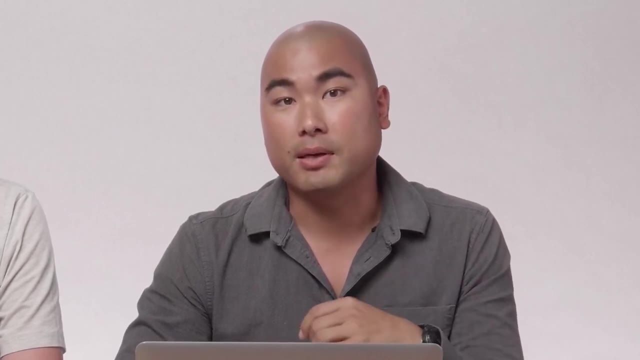 we call inbound data and a sync outbound data. when you bring data in, it becomes a collection in which a pipeline of operations, which we call transforms, can be performed. the data source can be batched or it can be streamed and there is a time windowing concept which allows for great 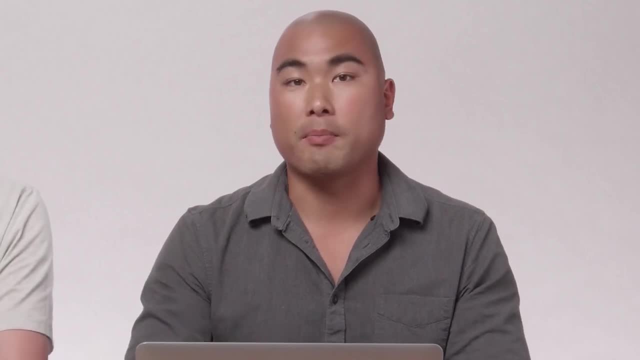 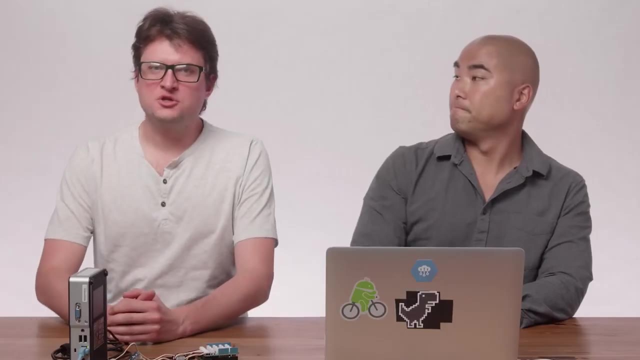 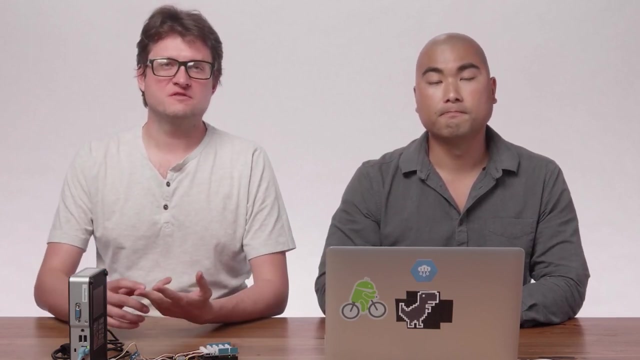 extensibility. you do all of this under a single programming model, which reduces complexity. before we go to a demo, gonna throw it back to Martin to talk a little bit more about ETL, sure? so there's gonna be three main parts of data handling that the Gateway does for us: uh, the extraction, transformation and loading. 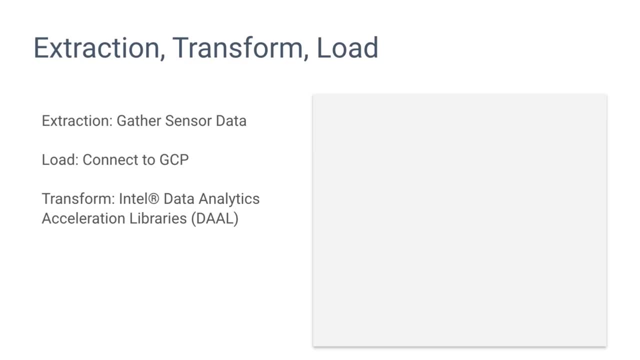 of data, or ETL as it's referred to in data science. we discussed the extraction of data, or gathering the sensor data. we talked about the loading of data, or ingesting it, into Google Cloud platform. now I want to talk a little bit more about the transformation of the data. so raw data is going. 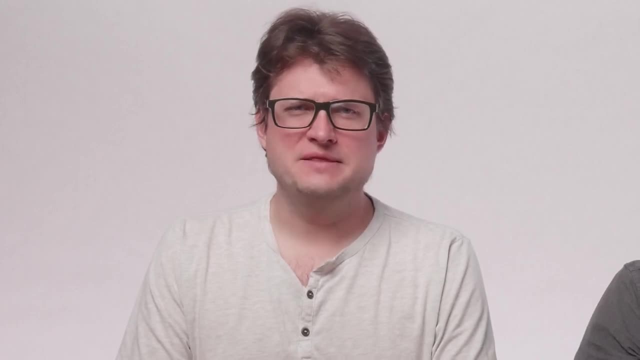 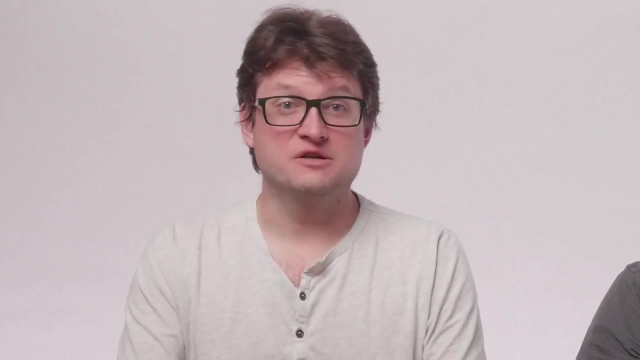 uh, there's going to be outliers, there's going to be some noise and there's going to be a time series of data that follows certain Trends. when we're dealing with a massive amount of data as a large scale industrial deployment, will we want to be able to clean that data up as fast as possible. 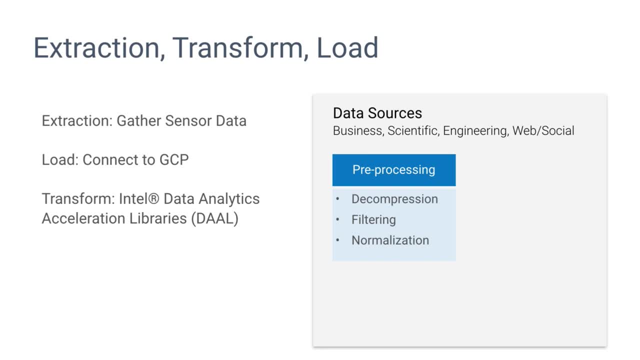 so to facilitate this process, Intel has developed a set of libraries called the data analytics acceleration libraries, or doll. these libraries cover a vast amount of data transformation methods, detection and low order moments or things like. means, sums, standard deviations. so these are just a few of the core tools that a data scientist can use to transform raw data. and all of these tools. 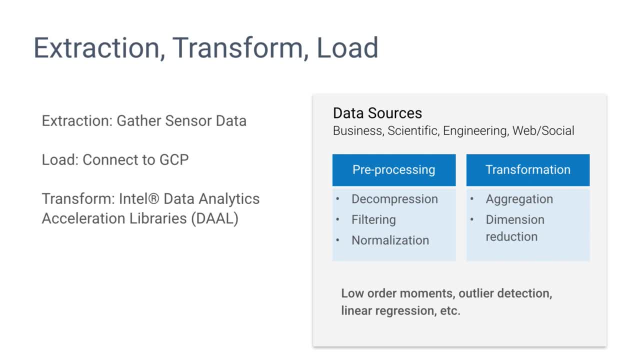 and many more are provided by the doll library, and using that, you can transform your raw data into something more usable. they they can then be fed into our cloud analytics pipeline, so these libraries have been optimized to run on Intel architecture in order to provide an extremely fast way to transform large amounts of data. and the best part is that doll runs on Hadoop, spark R and. 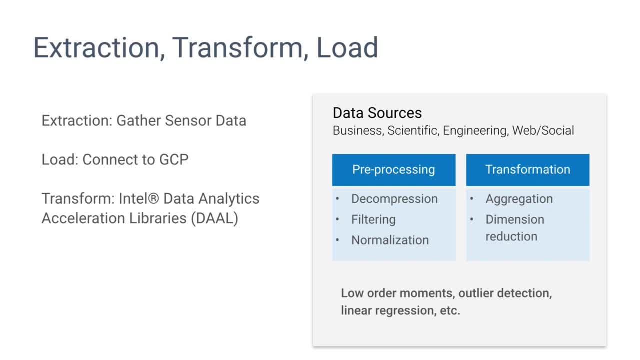 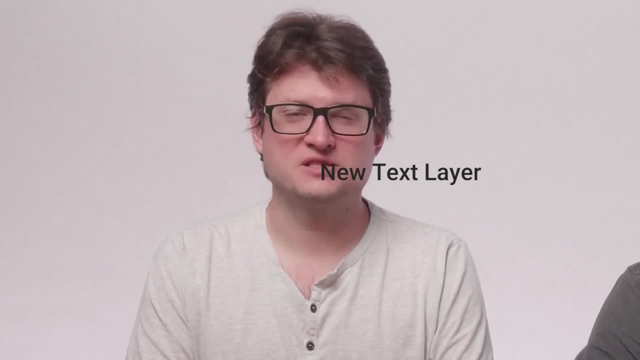 matlab. so that means that you can use the data processing pipeline with which you are most familiar with. if you want to try out these libraries for yourself, go to softwareinternetcom Intel dash daal to download the libraries, read about how to use them and try them out. 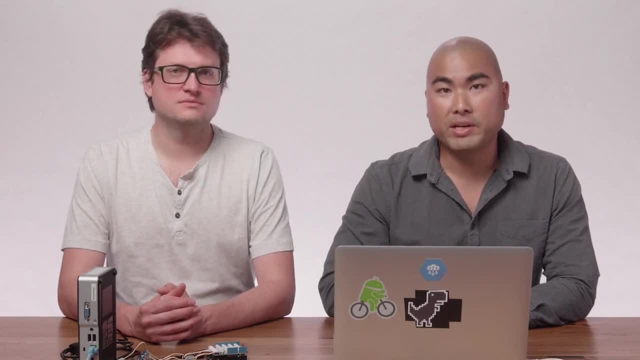 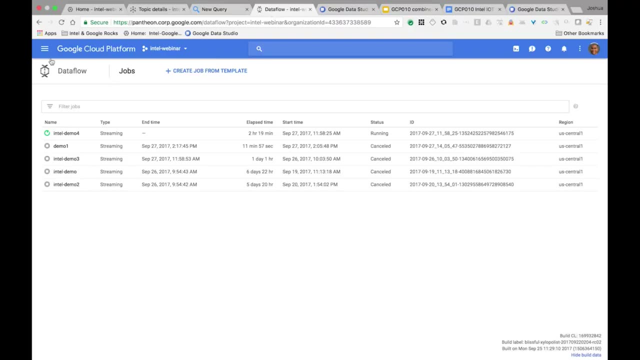 now that we have the e-tail performing on the Intel device itself, we can still use data flow to transport the data from pub subtopic into BigQuery. let's see how to get to date cloud data flow. you click on the hamburger menu and click on data flow. you notice I have a. 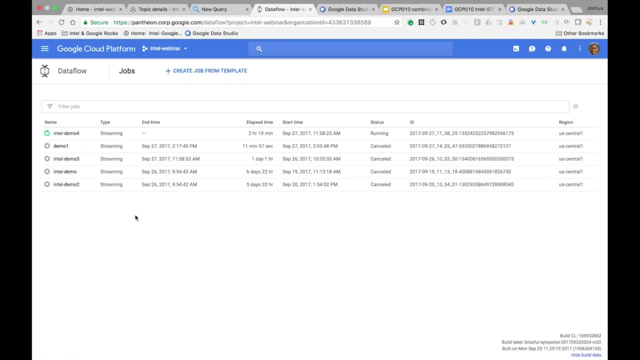 number of services already running this particular pipeline is running. to take the data from this device, from the topic and into BigQuery to create a new pipeline, I simply create a job from template now this we're using a template here because we don't have to do anything sophisticated here. 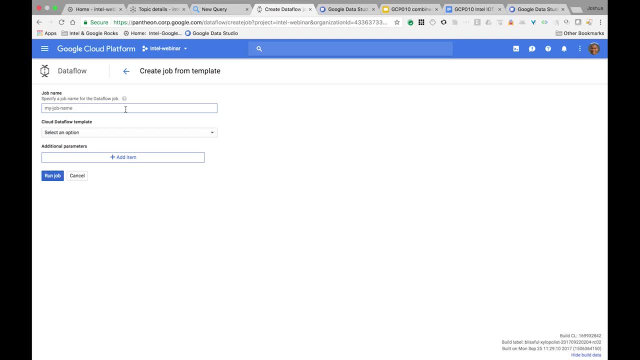 because the the nook here is going to handle the etl- I give this a name. I'm going to use the third option, which is cloud pub sub to BigQuery, and after selecting this option, I'm going to select two more. I need to provide two more pieces of. 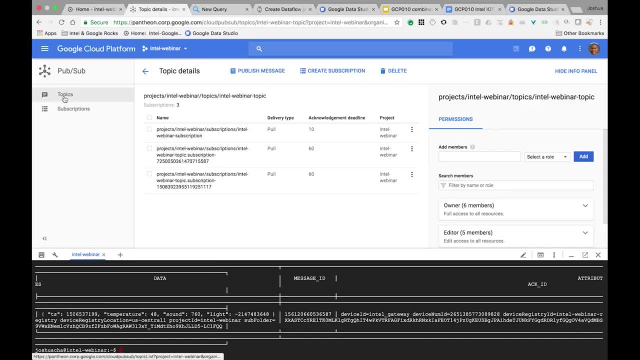 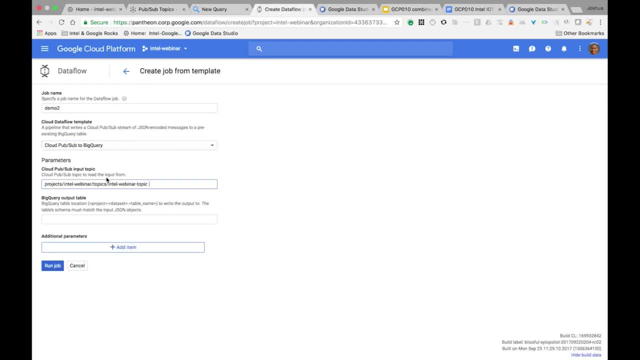 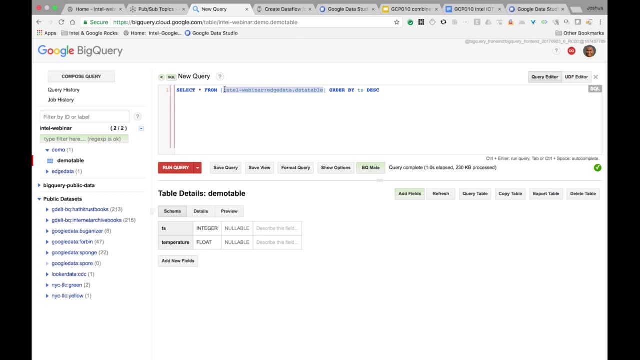 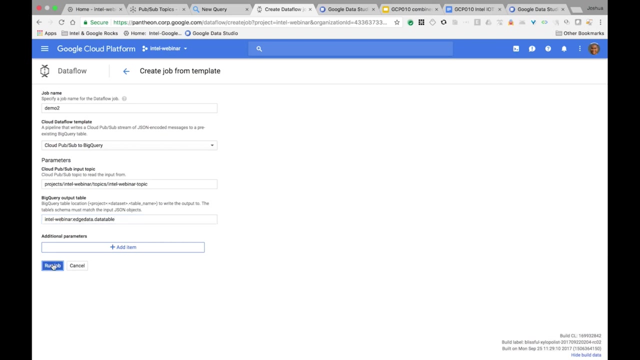 detail. one is the actual topic. since I have my pub sub topic already open here, I'm gonna select this topic and from BigQuery I'm going to select this table. now you know why we skipped over cloud data flow and went directly to BigQuery, so we. so, now that we have the BigQuery table defined, you click on run job and there you go. 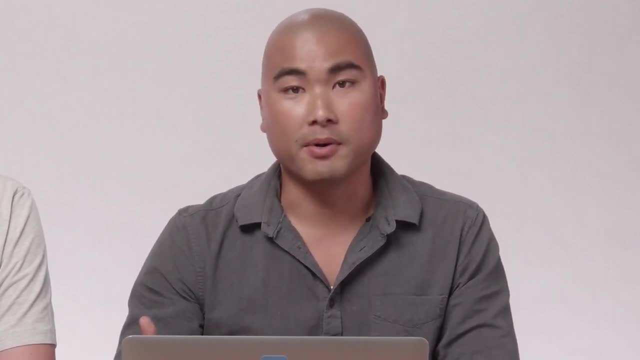 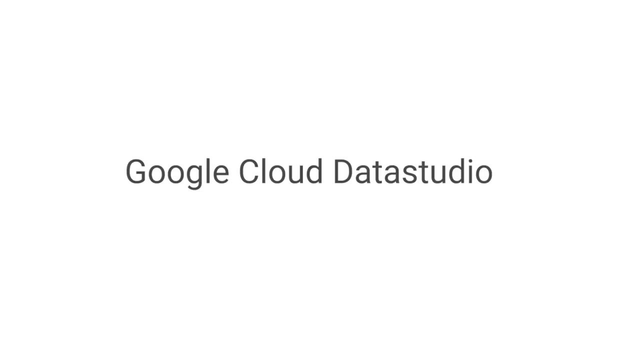 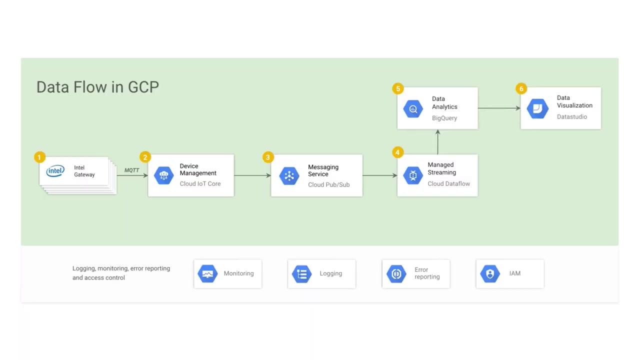 that's your first cloud data flow pipeline, taking data from a pub sub topic and into BigQuery. at this point, we've covered a lot of ground, so let's quickly review what we've done thus far on our data journey. we started out with the censored information coming to cloud IOT core. 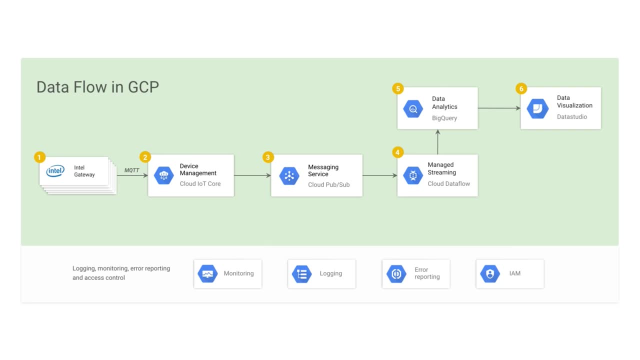 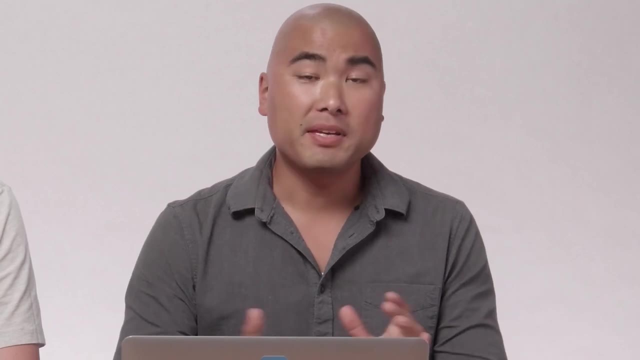 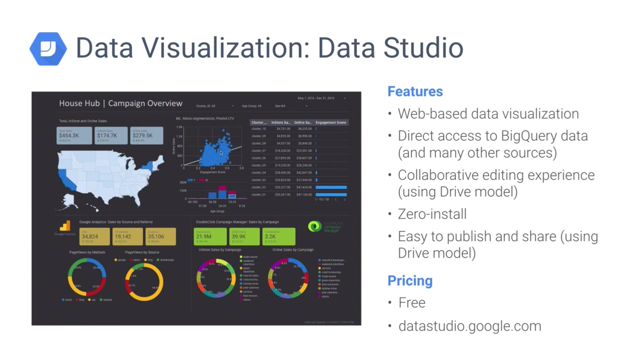 from there, the data got into a pub sub topic just now. we create a pipeline to take that data from the topic and into BigQuery. now, with the data in BigQuery, we can move on to the last step, which is using cloud data studio, which is a free tool that allows you to make beautiful charts from 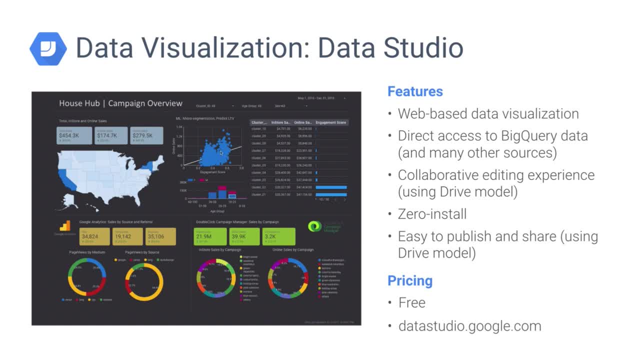 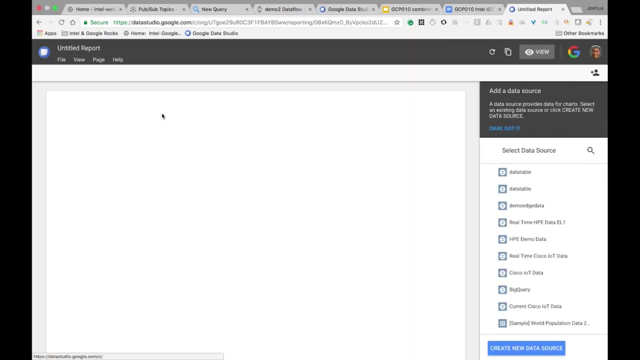 your streaming data. instead of me talking, let me walk you through a simple example. to get to data studio, you simply go to datastudiogooglecom to start, click on the big blue plus button to start a new dashboard. the first step when you create a dashboard is to create your first data source, in this case, 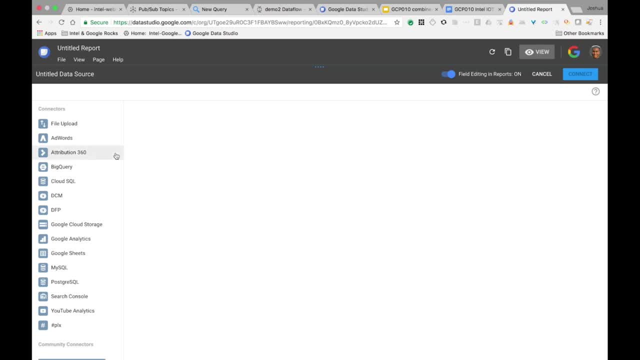 I'm going to create one from my GCP project. you click on this big blue button and you notice that data studio offers a number of data connectors. this makes it easy to connect your data sources. in this case, we're going to use BigQuery, because I've logged in with my GCP account and knows which. 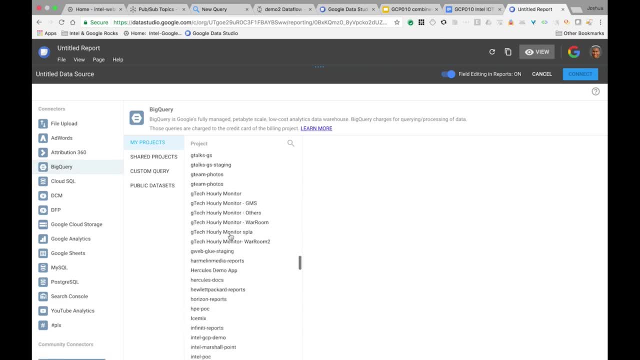 projects I am. I have access to. in this case we will be connecting with to the Intel webinar project as appropriate. click on Edge data and here's that demo BigQuery table we created. but here's Edge data Data table and I'm going to click on connect and connect this data source. 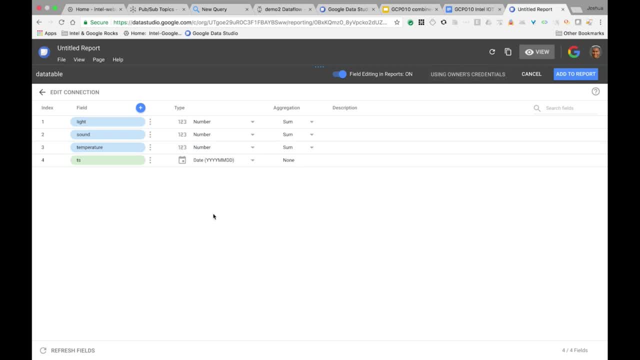 which you'll notice here is that I didn't code up anything. what data studio did was looked into that BigQuery table, found the columns and automatically created these metrics for me. it was smart enough to identify that light was a number, stress was a number, temperature is a number. even the time stamp which is specified as a number, even the current number is an hour and that's what Data Studio did and I'm going to click it. what Data Studio does is identify information in here which is getting a number now and we can show everyone the data sources we want, all the properties and the definitions that we created. we can see and show to you over here. if I wanted to worldview, And I'll let datacom you in to capitalize I think thatникомus as one or two pieces data, but we are now at the date- solid data and that's the data table. we're doing this project and 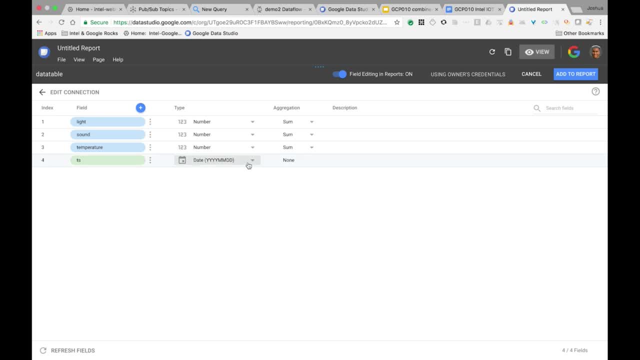 integer. in BigQuery it was identified as a date, which is correct. Here I'm going to change a few parameters around. I'm going to make these averages instead of sums And let's add a bit more detail to the time here, to include both the day and the hour, just to make it a bit more interesting. 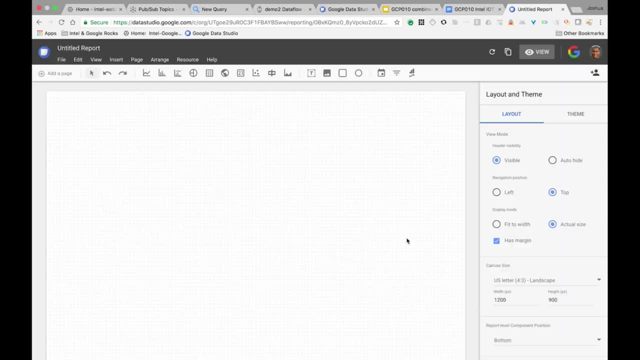 I'm going to add that to the report. Okay, and here's your first dashboard. Let's create a table that just takes the raw data and dumps it to the screen. To do so, I click on this table icon. draw the table in the dashboard. 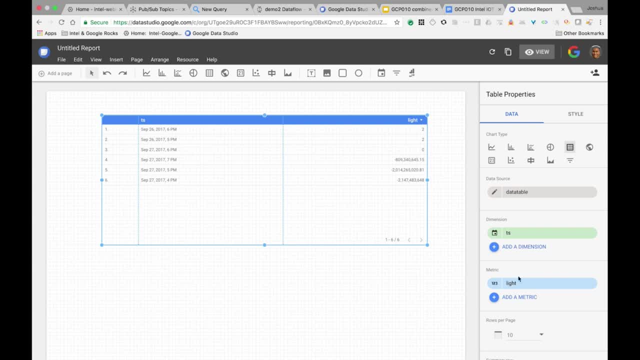 And you'll notice immediately. the timestamps are already populated here. It added light, but we could add a couple other metrics. Let's add sound And lastly, let's add temperature. And there you go. So now you have a data dump. 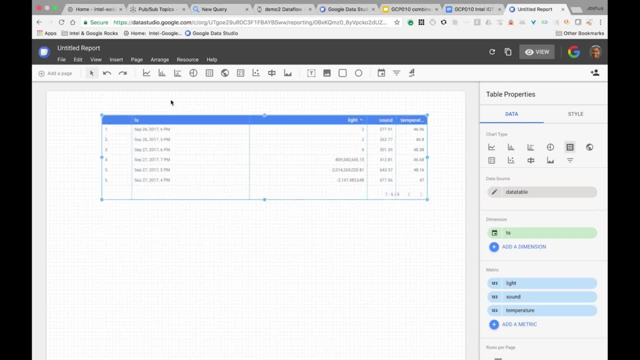 the information coming in from the sensor. Let's create a chart now to make it a bit more attractive. So I'm going to start with this time series chart. It's essentially a line chart. I'm going to drag into the dashboard And you'll notice that on the x-axis it'll automatically. 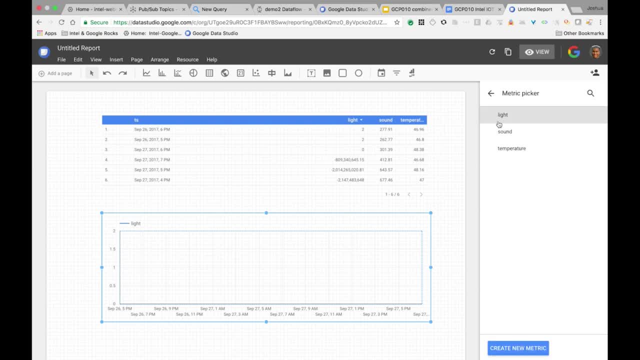 populate it with a timestamp. By default, it's adding the light, but we could add the sound, And let's also add the temperature. And there you have it. In about five minutes we created a beautiful, beautiful table with all your data and a chart that gives it a bit more meaning than just. 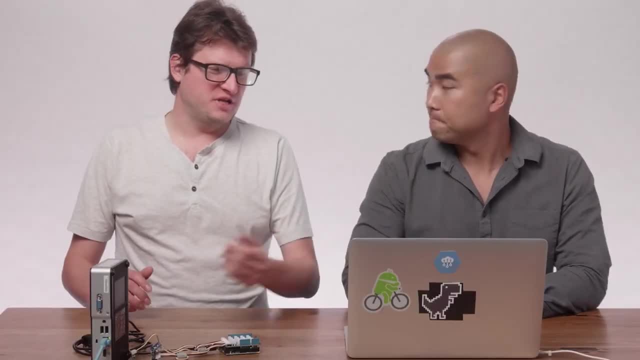 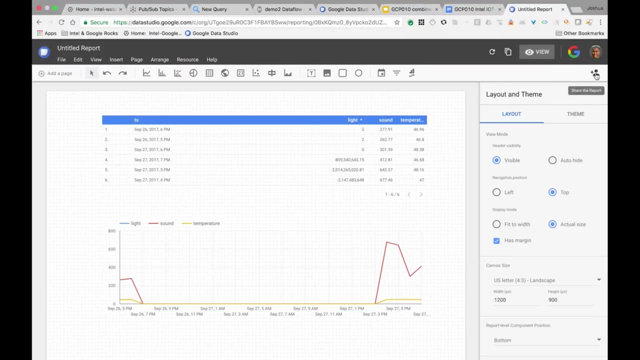 a list of raw numbers. Yeah, so this visualization looks really great And I'm guessing that you can easily share it with other people on your team. That's right To do so. you just click on the sharing icon and list your teammates that you want to share it with. That's it. 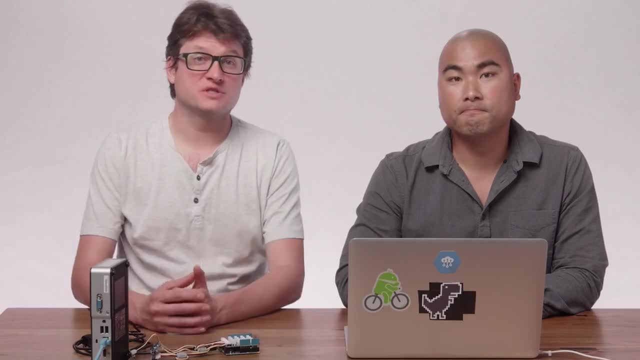 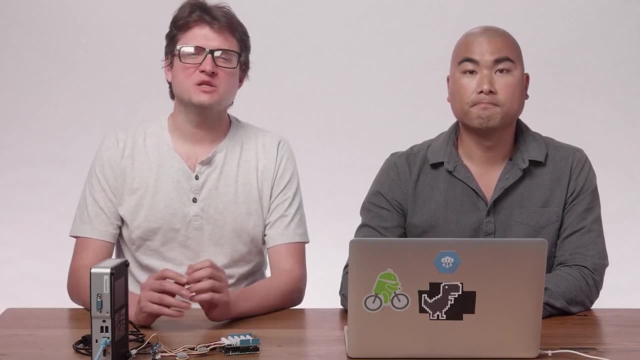 Great. I mean, this looks really good And I can definitely see how developers can use it to start pulling out business logic from their data. Before we sign off, I just wanted to circle back and discuss a little bit more about how we can use this to start pulling out business logic from their data. 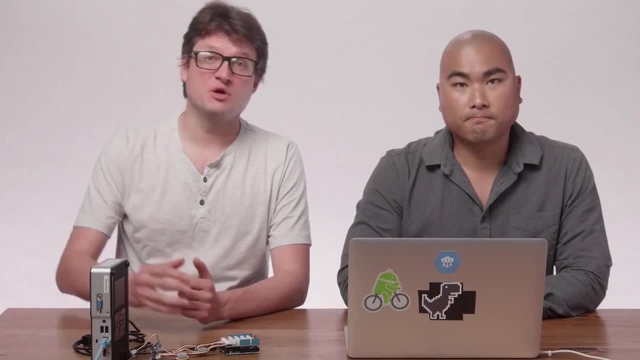 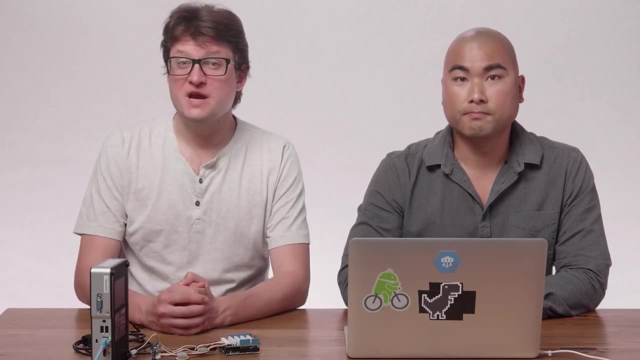 So let's talk a little bit more about advanced analytics that you can do on the Intel-based gateways. So the type of data that we're able to visualize here, and really in almost all cloud-based frameworks, is limited to what you can send via JSON, So numbers like floats or integers. 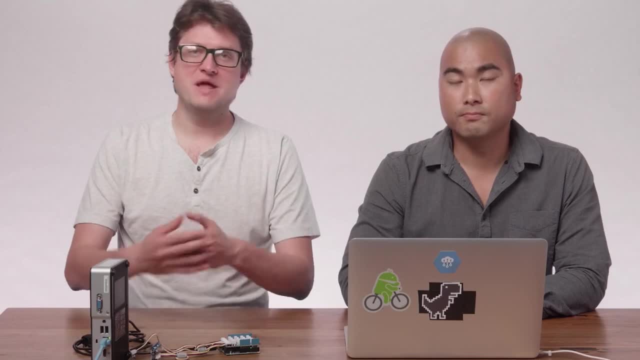 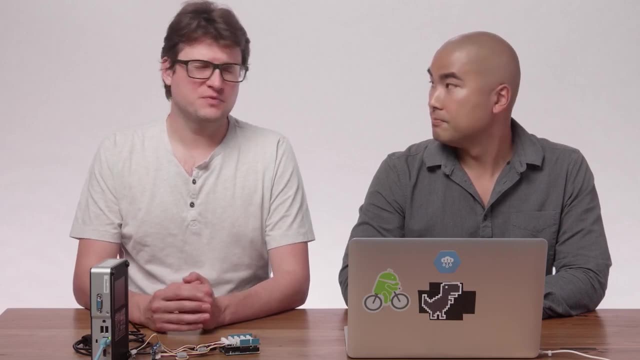 and strings of characters. This works great for many data applications. Our demo here uses sensor data which is encoded as an integer value between 0 and 1023, which is a pretty standard way of doing analog-to-digital conversion. So let's talk a little bit more about how we can use this to start pulling out business logic from our team. 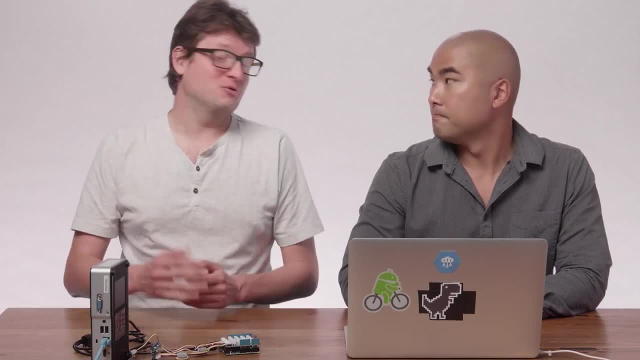 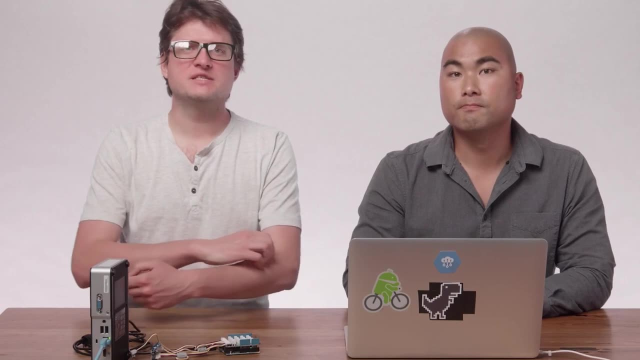 But what if the data that you're gathering can't be encoded into a number or string? So, for instance, more and more applications are based around gathering video or images, And the only way to send an image with a JSON would be to break it up into an array of pixel values. 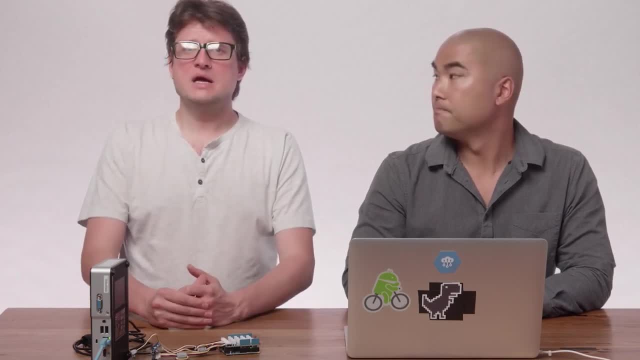 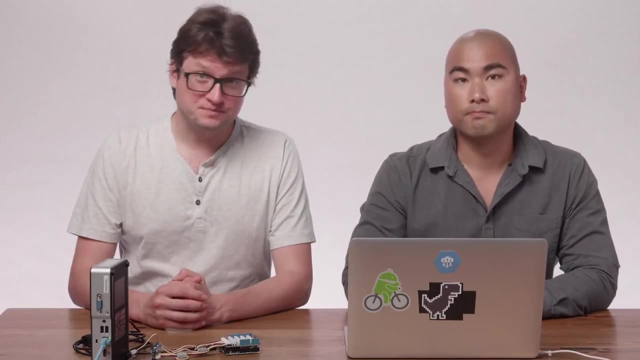 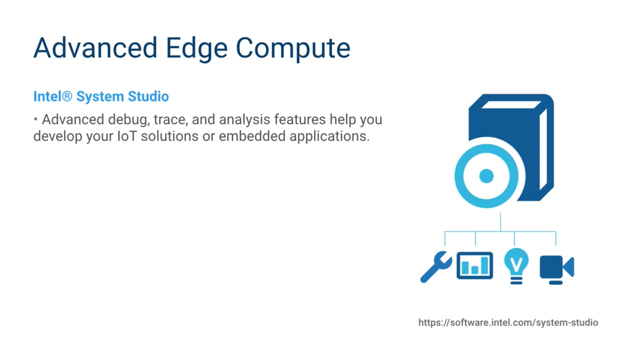 And this can be both cumbersome and very bandwidth-intensive. So what you need to do then is some kind of advanced analytics at the edge before you can send that data up to the cloud. So Intel provides a whole host of tools for just that with the Intel System Studio. This is an IDE for C++ that integrates a whole host of libraries. 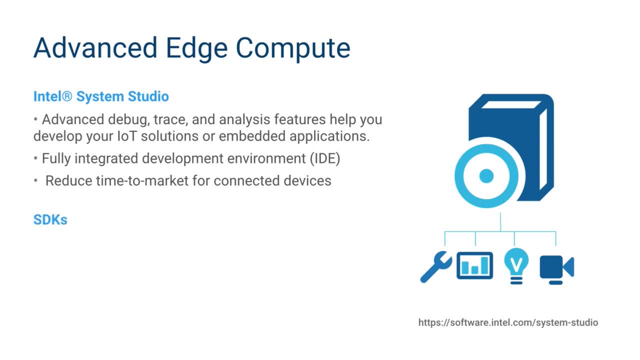 and SDKs, which are created by Intel and meant for advanced analytics. Check out softwareintelcom slash system dash studio to learn more, download the IDE and just start using it and applying it to your projects, One of the tools that's included in this package. 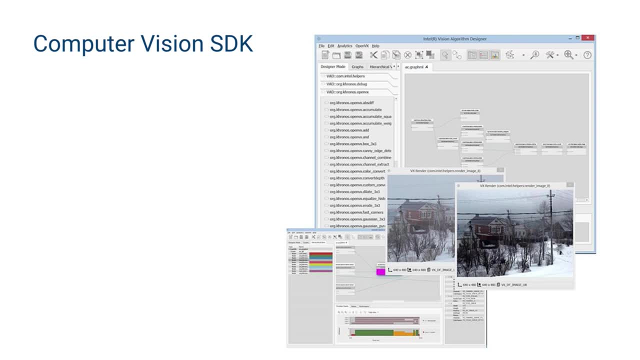 is the Computer Vision SDK. So this SDK was released into public beta about a month or so back and integrates a bunch of really useful tools for computer vision applications. It's based around OpenCV, which is an open-source project for computer vision. 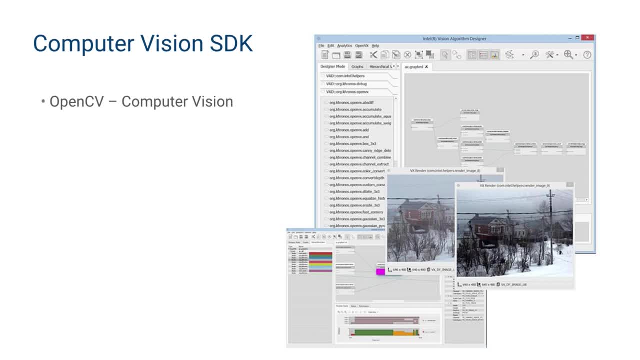 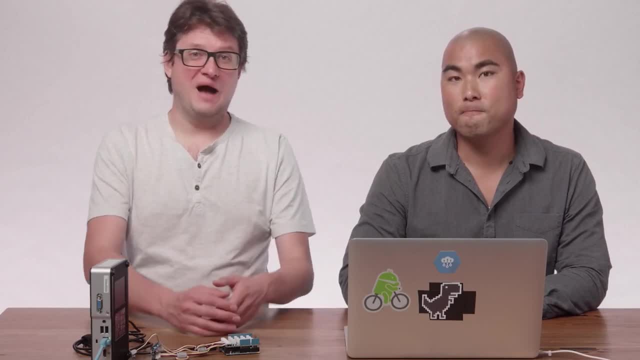 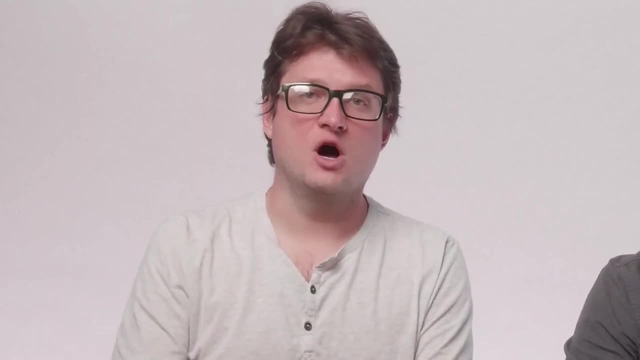 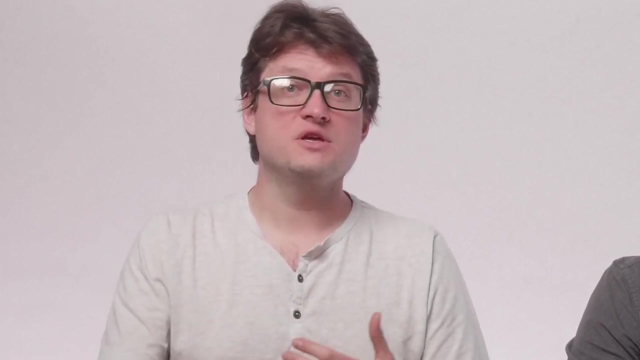 So what does this mean in terms of our data flow? Well, it means that, instead of sending up an entire image, you can analyze it with the CV SDK on the gateway and then send a data format that's easy for our pipeline to ingest, And in this way, you can expand the kinds of data that you can use. 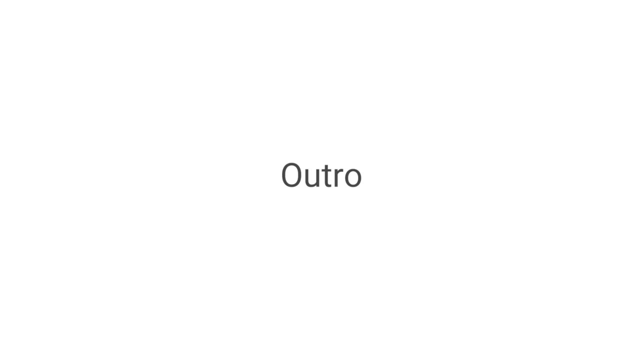 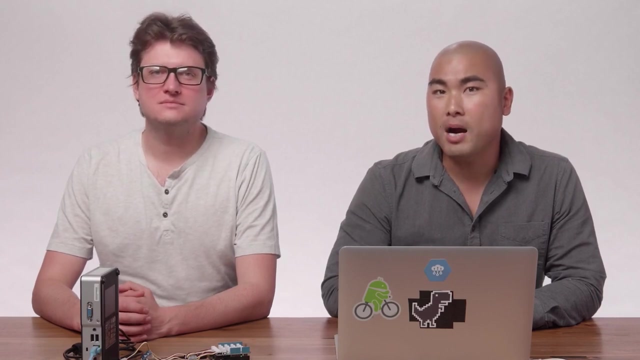 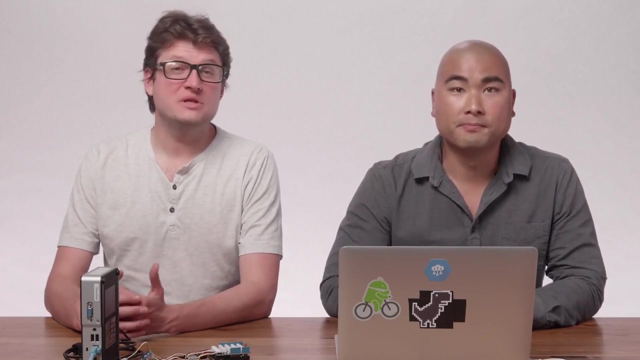 in your application. That's all we have for today. We hope that today's session shows that, with the combined power of Intel's hardware platforms with Google Cloud, you too can build a highly scalable, reliable data pipeline. And please stay tuned for our next webinar, in which we're going to 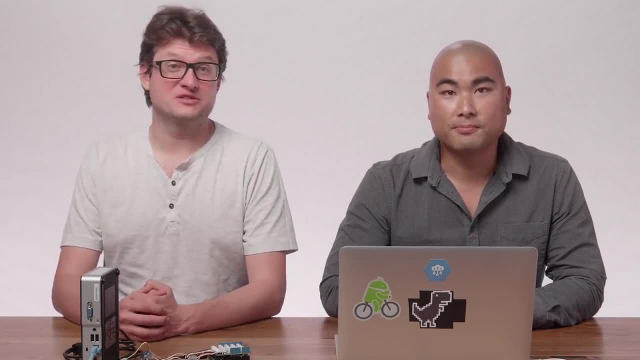 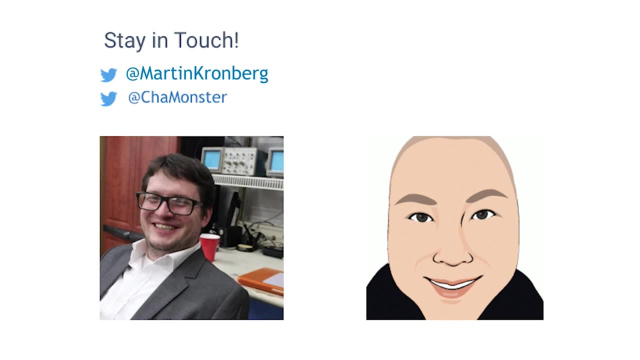 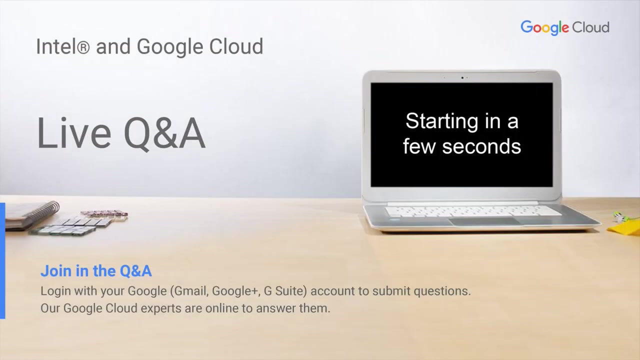 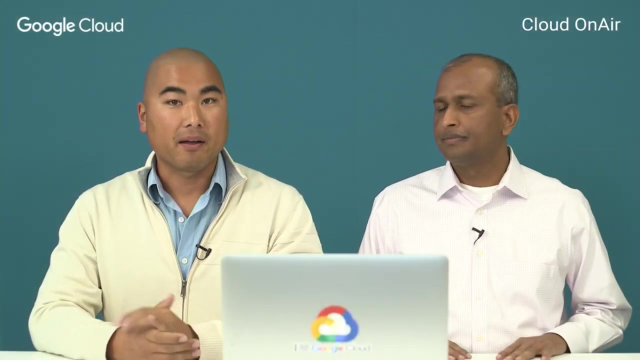 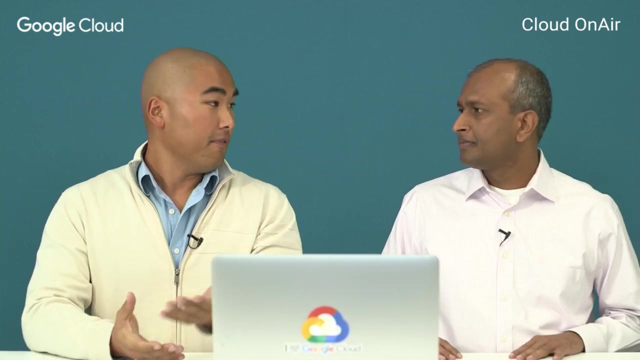 demonstrate how you can use this data to build your own machine learning solutions. Thanks, guys, Welcome back. We hope you enjoyed the presentation And thank you for your questions. We've gathered a number of questions that we hope we can answer. To start off, let's start with number one here. 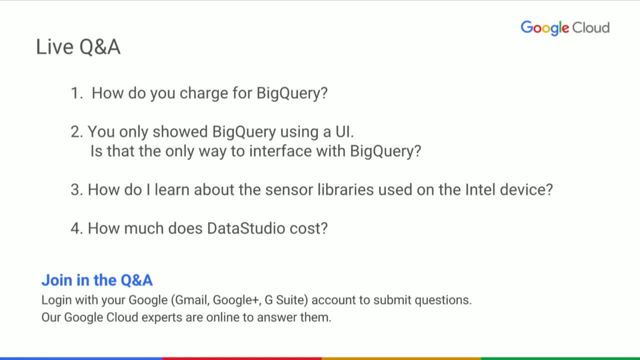 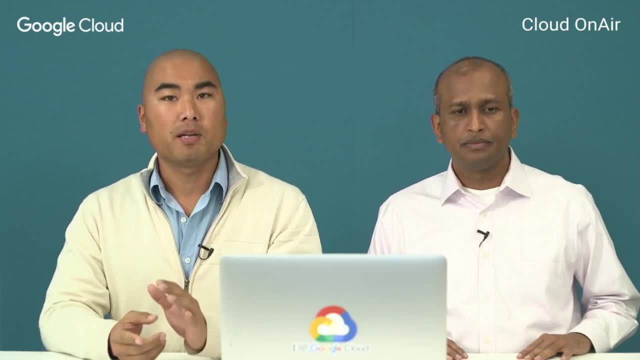 How do you charge for BigQuery? Now, there are three dimensions to BigQuery pricing. The first one is storage, the second one is streaming and the third is the query. On the storage side we charge about $10. You can charge about $15 for BigQuery and you can charge about $20 for BigQuery. 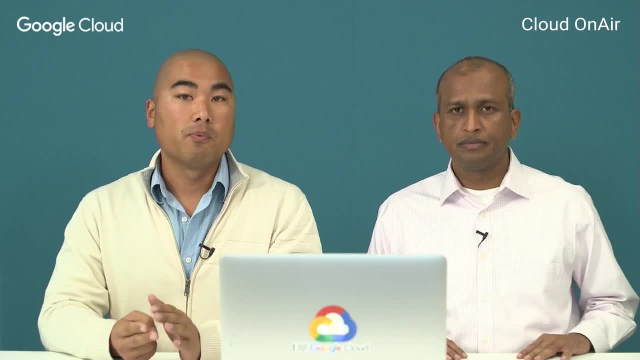 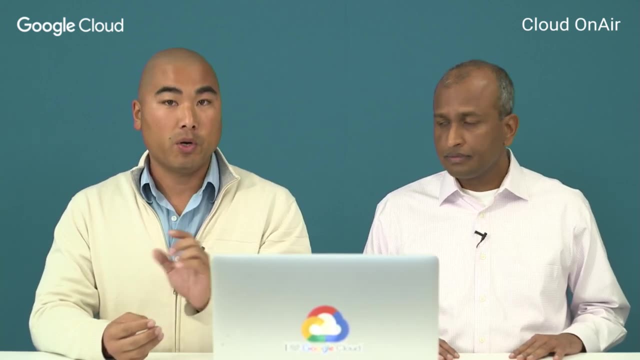 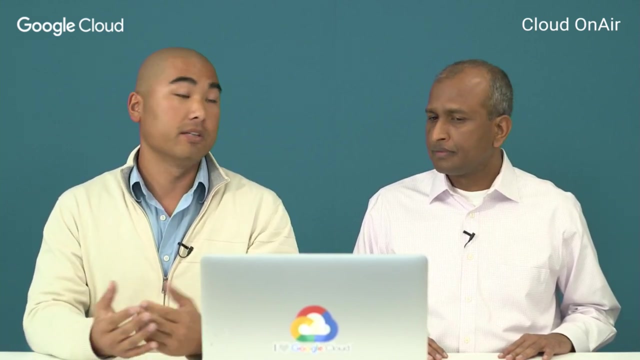 On the streaming side we only charge a cent per 200 megabytes per month And on the query side it's $5 per terabyte of query, with the first terabyte being free. Now data coming into BigQuery and data coming out of BigQuery is free. So if you have any questions, there's more information. 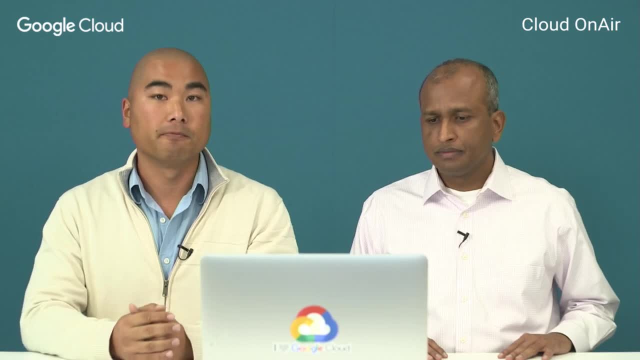 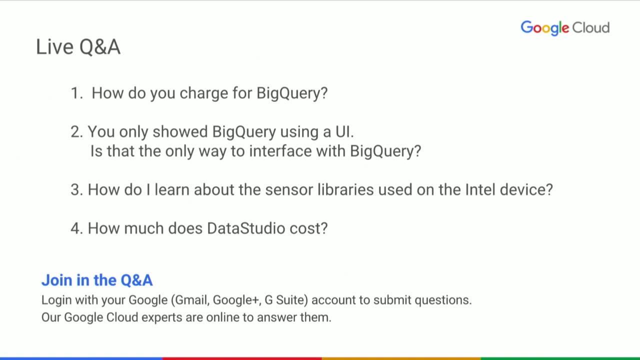 on the website under BigQuery in the Google Cloud Platform website Number two, another BigQuery related question, You only show BigQuery using a UI. Is that the only way to interface with BigQuery? The answer is no. There's multiple ways. 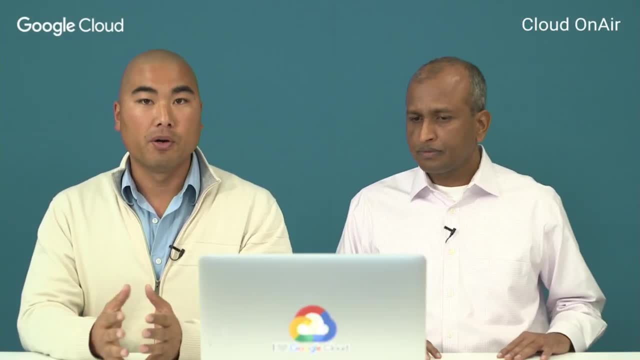 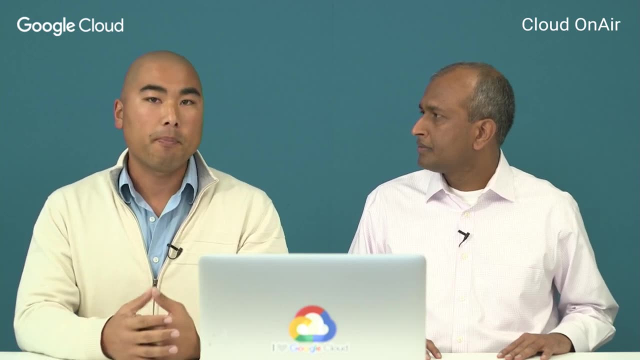 The first way is through our REST APIs, very well-known REST APIs. The second way is through our gcloud command line interface. The third way, and I would say the most popular way people are interfacing with BigQuery is through our native APIs. So we do have APIs built for Python. 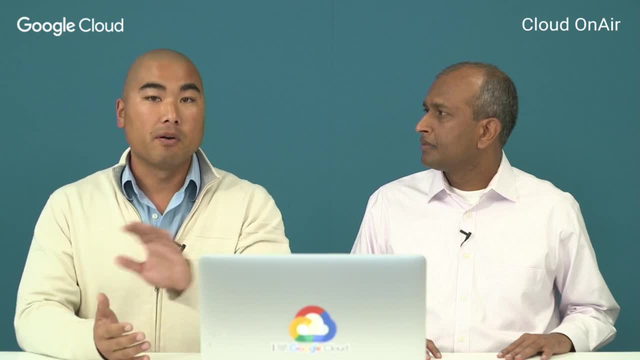 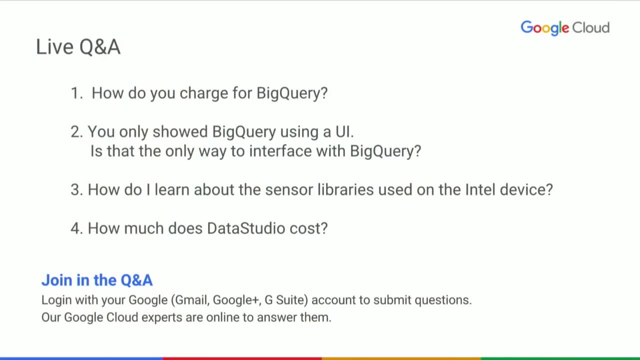 NET and Java. So as a developer, you have your options on how you want to leverage BigQuery into your project. Cool, Here's a question on sensor libraries. So the question is: how do I learn more about sensor libraries used on the Intel device? So Intel actually maintains: 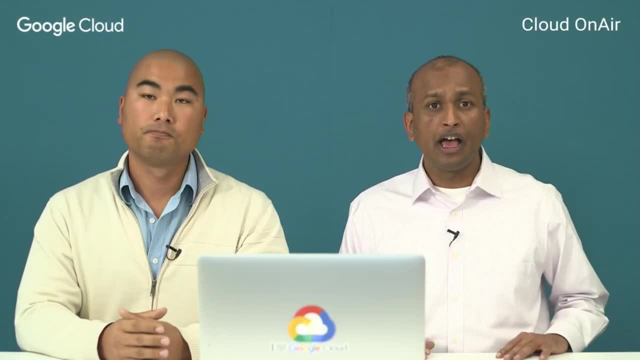 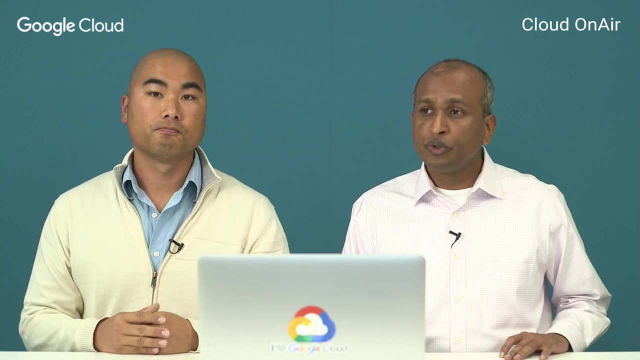 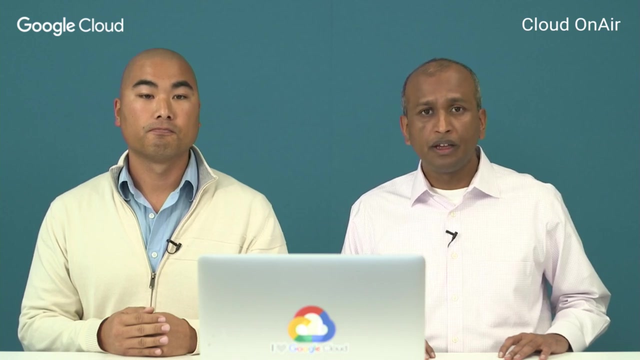 a website called upmmraaio. It has all the information about the sensor libraries, the APIs, which sensors you could use. This site was recently revamped so you should be able to use it. It should be easily accessible. Again, the website is upmmraaio. 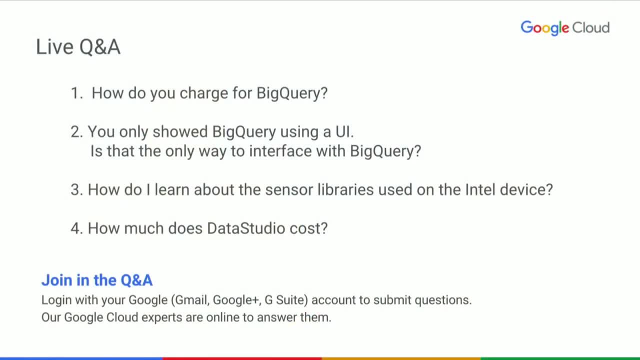 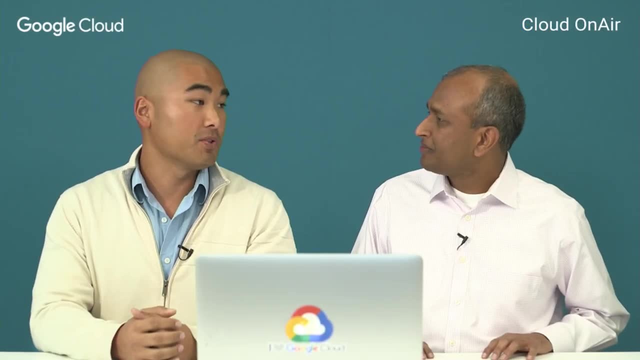 Great. Thank you, Sundar. Number four: how much does Data Studio cost? So there's a theme here. Developers are concerned about cost. The good news about Data Studio is that it's a free product as the date of this recording, And it's currently in beta, so it's a free product. However, I do 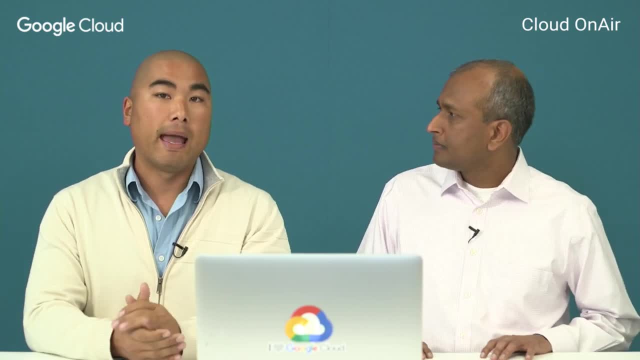 want to inform our developer community out there that if you're using BigQuery as the data store to serve the data and to generate data, you should be able to use BigQuery as the data store to serve the data and to generate data. However, I do want to inform our developer community out there that if you're using BigQuery as the data store to serve the data and to generate data, you should be able to use BigQuery as the data store to serve the data and to generate data. However, I do want to inform our developer community out there that if you're using BigQuery as the data store to serve the data and to generate data, 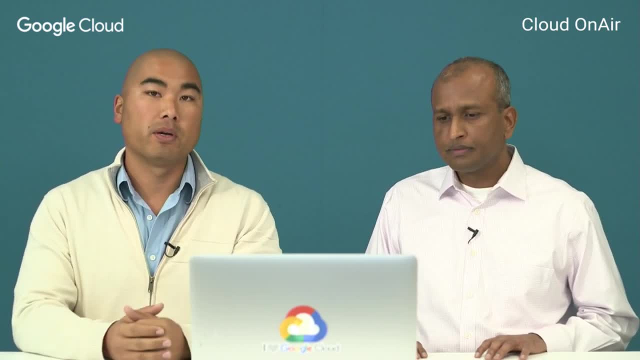 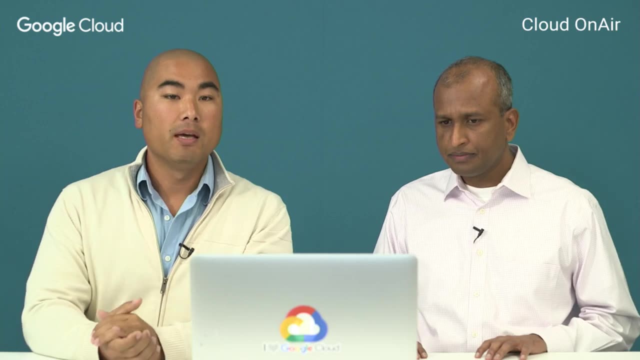 you will be charged for the querying and the storage of that BigQuery data. So watch that. But the product itself today is a free product. Cool, Let's see Again. All right, Great Number five, another Data Studio-related question. It's a. 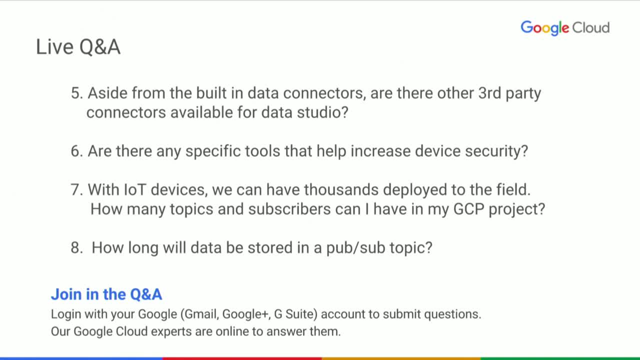 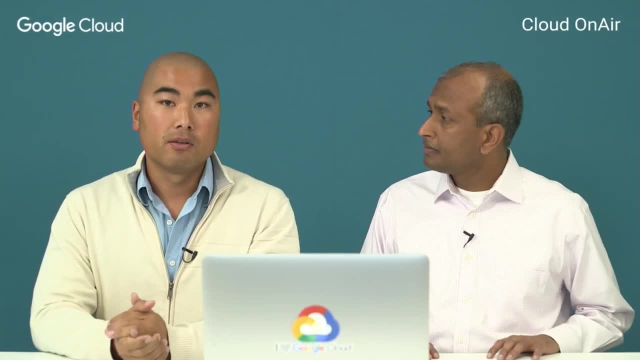 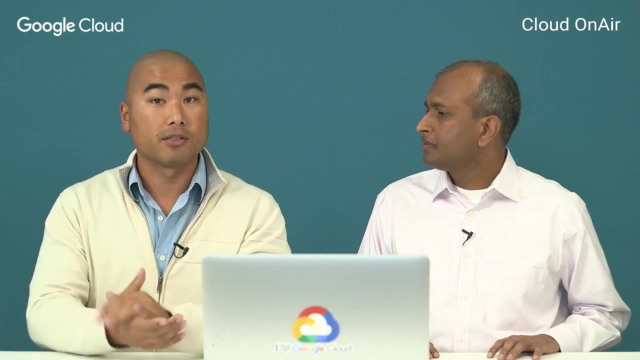 great question: Aside from the built-in data connectors, are there third-party connectors available for Data Studio? And the answer is yes. If you Google Data Studio community connectors, you'll get a result. The first result will be a page where we allow and educate developers to create their own Data Studio connectors. 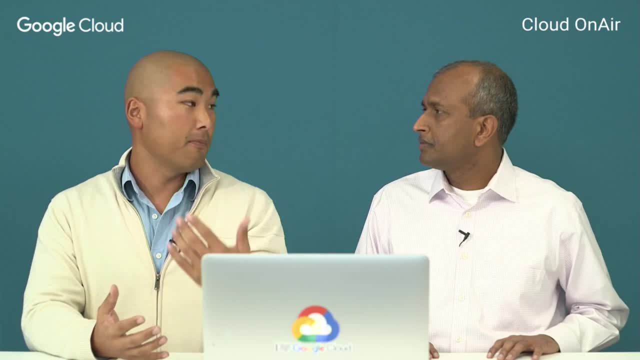 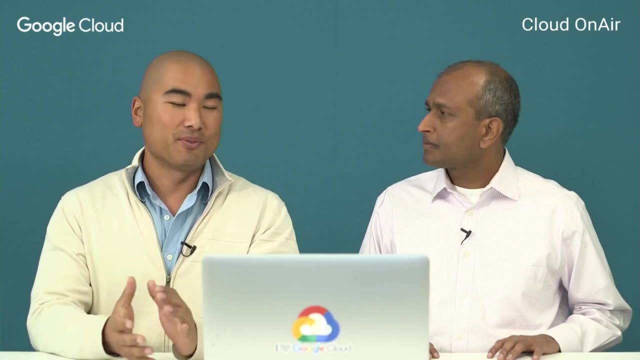 So if the standard built-in connectors don't do it for you, you build your own And you use a product called Apps Script, which is beyond the scope of this webinar, but it's pretty easy to pick up as well. There's tons of information online. 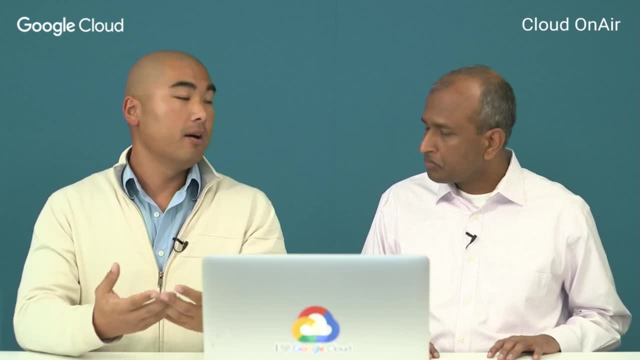 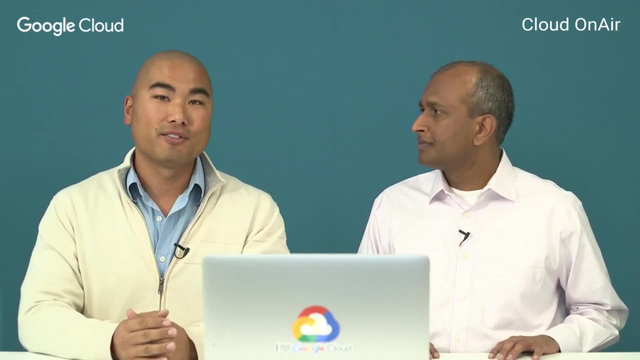 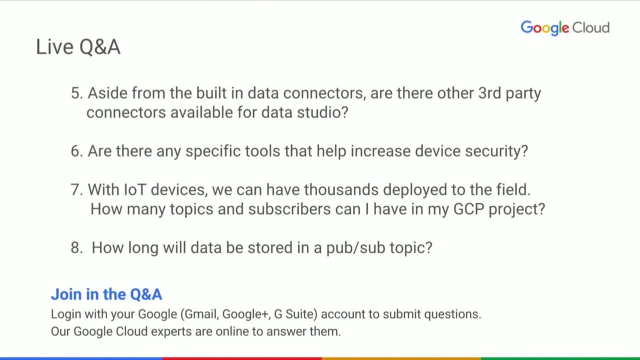 In addition to that community page, we actually have a gallery as well for third parties who have already created these connectors. That gallery is linked off this community page. So again, search for Data Studio community connectors- Excellent. Here's a question on device security. 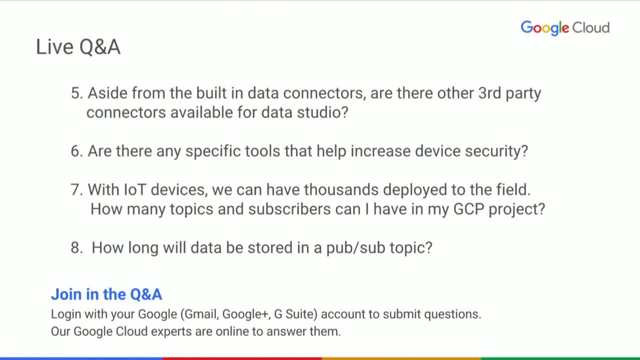 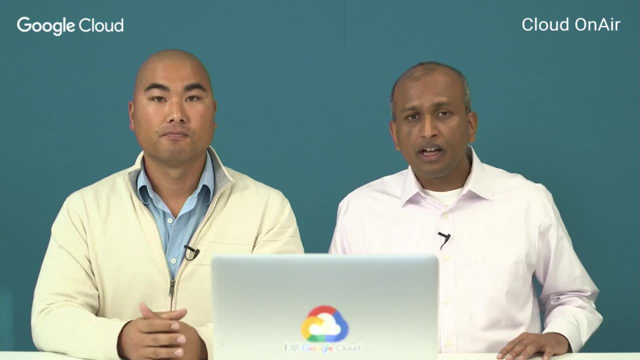 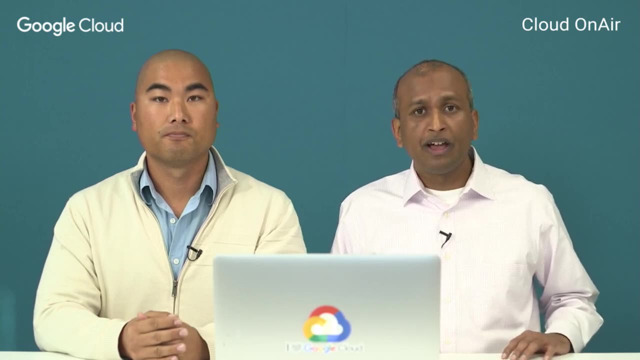 So are there any specific tools that help increase device security? Actually, there are In fact. very recently, at the IoT World Congress, we announced a specific feature called a secure device onboarding. Take a look at it. More information is available at wwwintelcom.